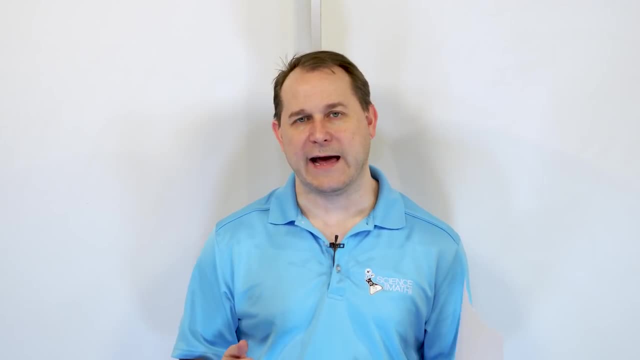 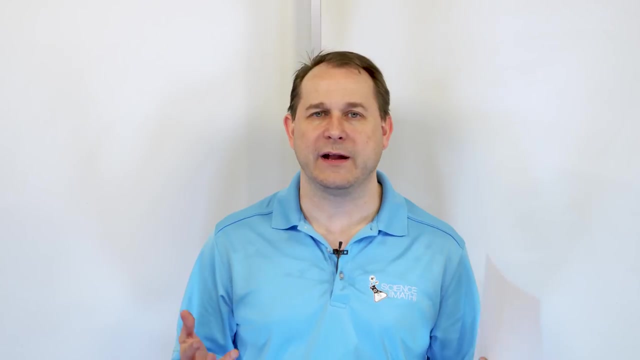 multiplying binomials And you're taught that in every algebra class it's the way that we multiply binomials together, But almost no teacher actually explains to you why we multiply binomials using that FOIL method, And I really don't like that because it tells you that hey, you have. 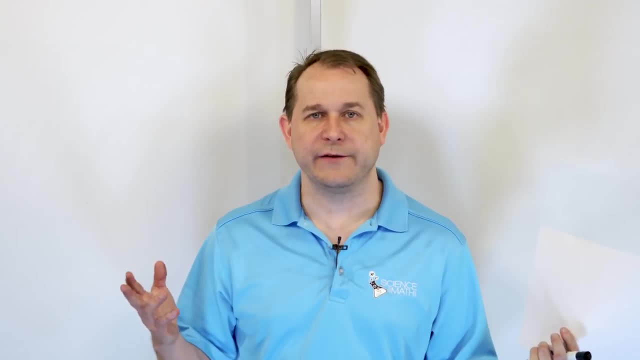 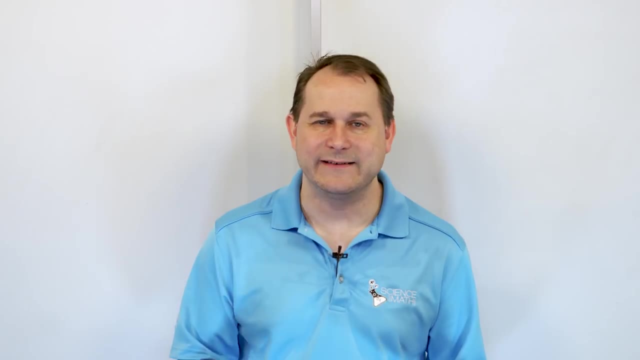 to memorize all these things that your teacher says and you just do it that way. and there's no reason. just do it that way, it's just the way it is. Well, the truth is, the FOIL method of multiplication makes sense, And I'm going to show you what the FOIL method of multiplication. 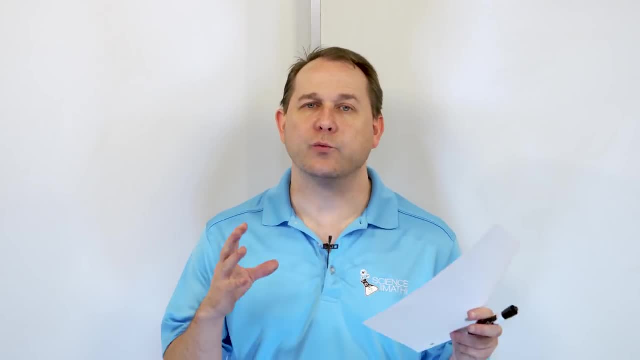 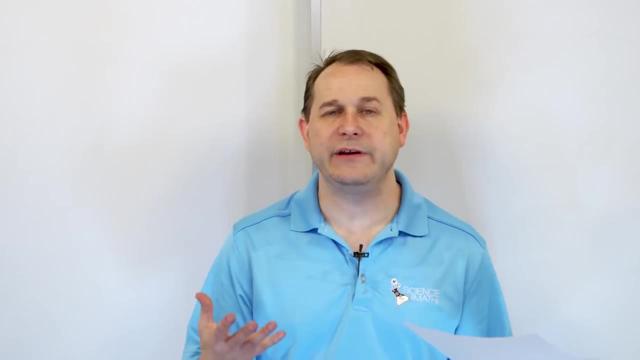 is what multiplying binomials really entails and why we use that method and why we use those letters. So at the end of this lesson you should understand how to multiply using FOIL and why we do it that way. And in the next two lessons we'll be getting more practice, two more detailed. 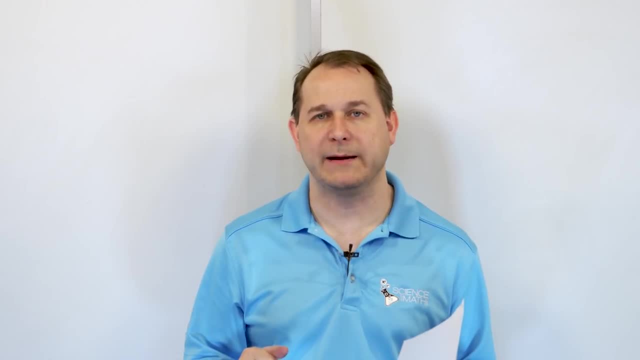 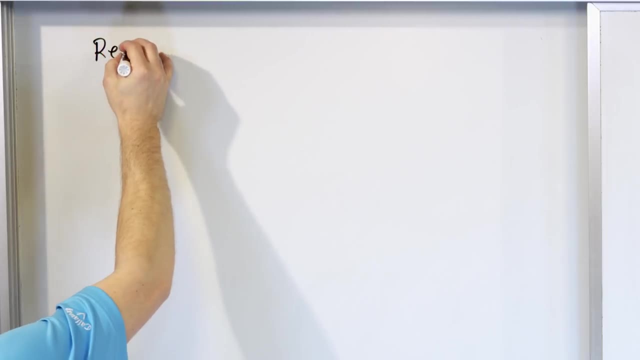 lessons of more complicated problems to give you practice multiplying binomials together. So, before we go any further, I want to recall- or have you recall- something that we learned in the past, Because it turns out that multiplying binomials is related to what we've already done in the past. What if you have x times something? 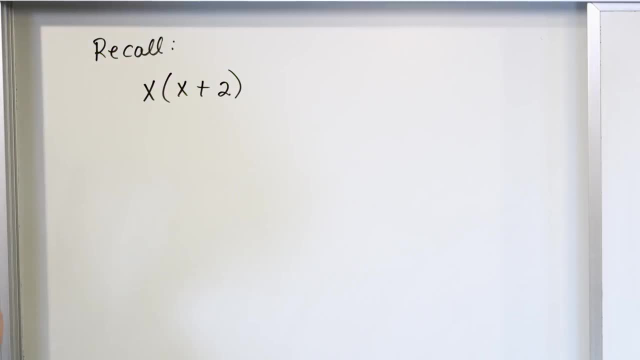 very simple: x plus 2?. How do you do this? So you learned a long time ago that when you have a term wrapped in parentheses, or two terms, in this case a binomial- this is a binomial, by the way. two: 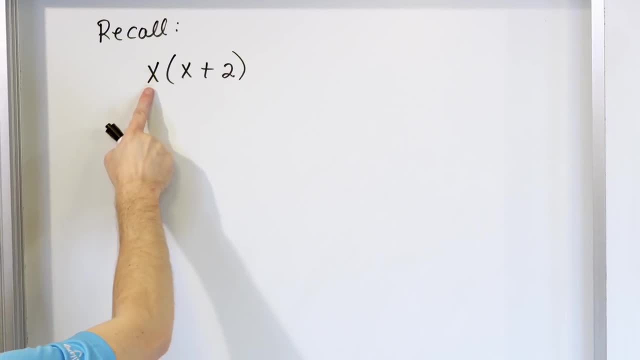 terms in parentheses- and you have something on the outside- this is a monomial- then what you do is you take what's on the outside, you multiply it times this term, and you multiply it times the other term, and then you write them out. So what? 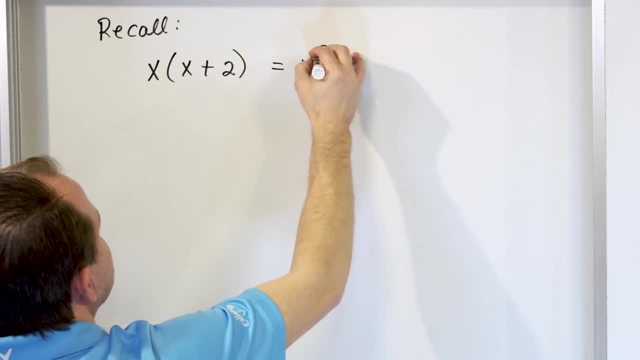 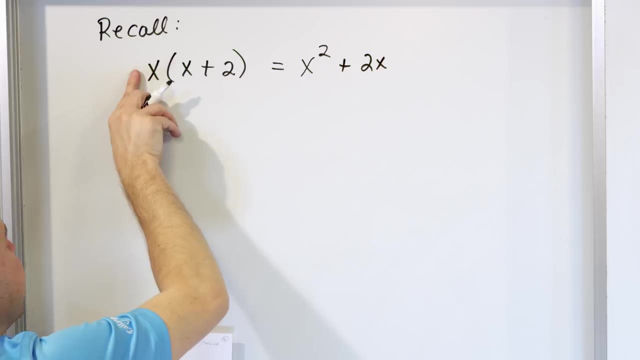 you're going to get is x times x is going to give you x squared, and then x times 2 is going to give you 2x, And the reason there's a plus sign here is because there's a plus sign here positive 1x. 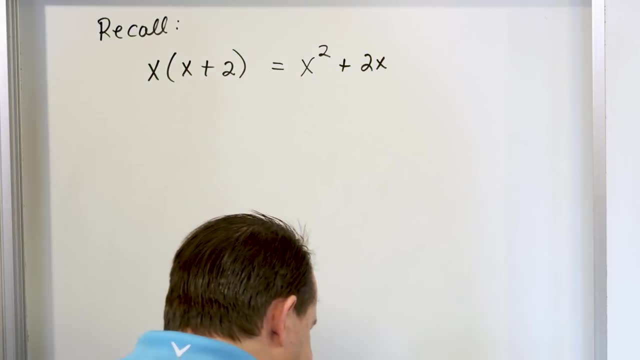 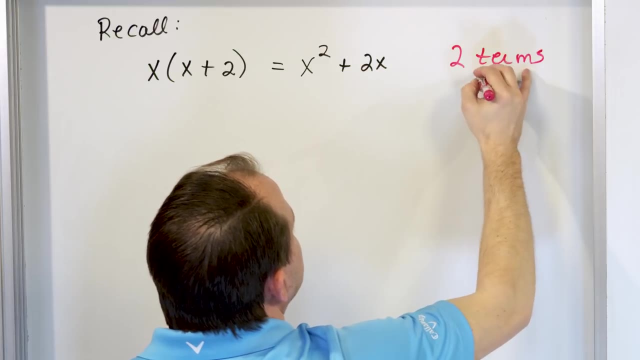 times positive 2 will give you the positive 2x. Now notice here that in your final answer there were actually two terms in answer. right, Two terms. This is number 1 and number 2, and that'll become interesting. later on I'll talk to you about it. 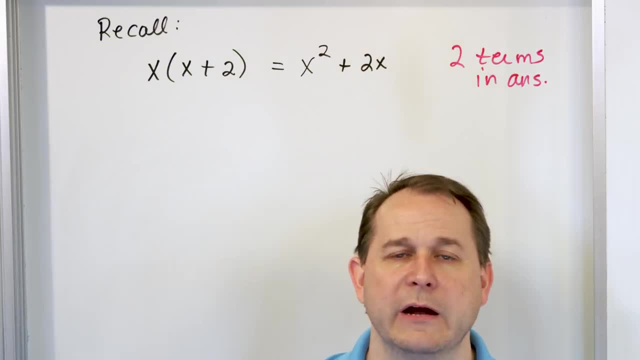 So the critical thing to remember about multiplying anything in algebra is when you have a parentheses, a set of parentheses with- in this case, we had two terms inside, but actually it can have any number of terms inside the parentheses, right Then if you have something sitting right outside that. 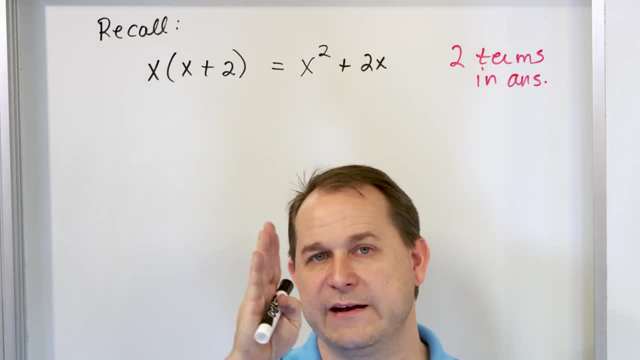 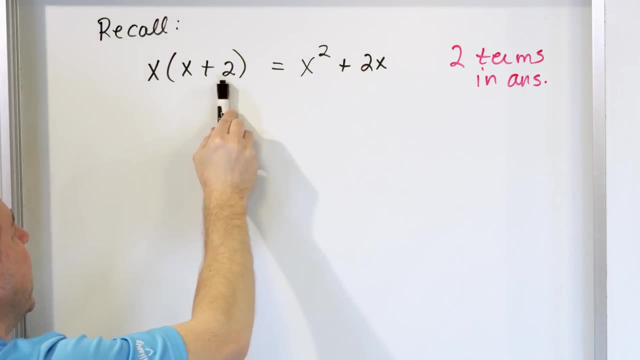 parentheses- then you know from the rule of distribution that in order to do all the multiplication you have to take that outside term and multiply it times every term on the inside, Because if you only multiply it by half the terms, then you've only done half the multiplication. 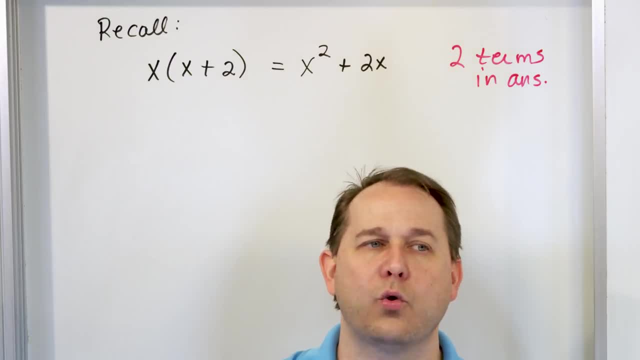 That term, inside the parentheses, consists of two things. So in order to do the complete multiplication, the outside thing has to affect everything on the inside, Otherwise you've only done half of the multiplication, All right. So anyway, you've done it via distribution. Now let's go and take. let's change it a little bit. 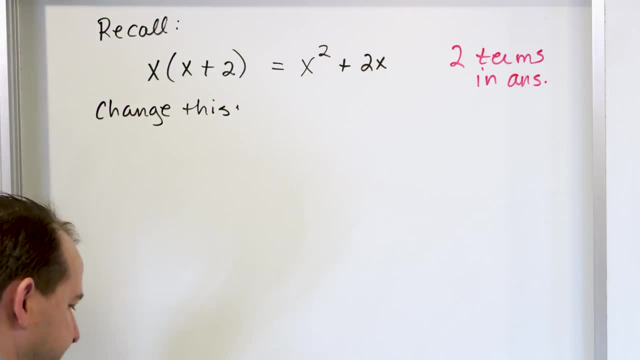 Let's change this to the following thing: Let's change it So that you have on the outside, instead of X, you actually have a parentheses with something like X plus Y, And on the end, on the other parentheses, you have X plus two. 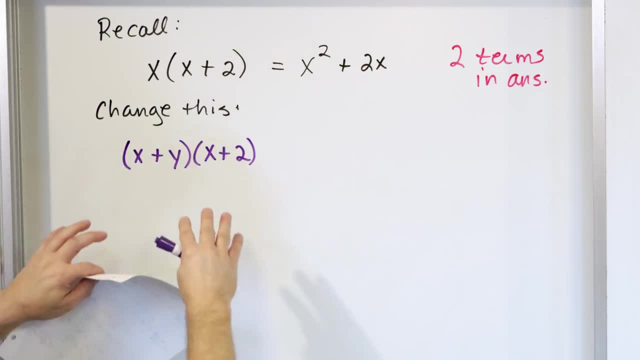 Now, for some reason- and I was the same way when I learned this- when a student sees this, your brain starts to go berserk and you have no idea like whoa, the alarm bells start going off and all of that. 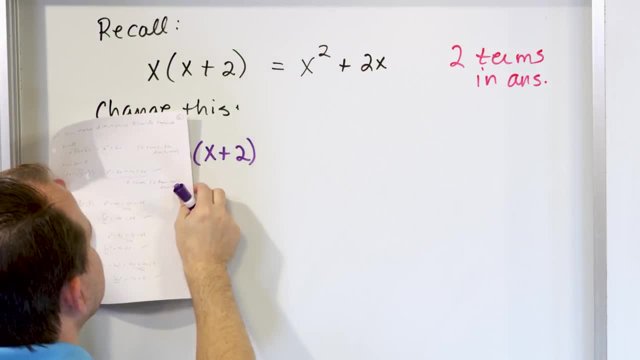 But when you think about it, what's going on here is you're still multiplying something by X plus two, just like you were doing here, And you know how to handle this. You take the X times this and the X times this and you add them together. 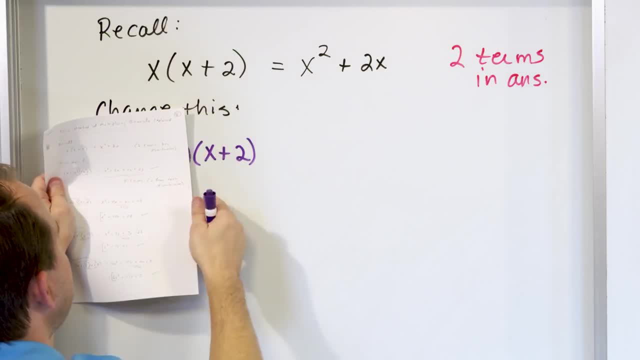 Right, But now, instead of multiplying by a single thing on the outside, we're just simply multiplying by two things linked together with a plus sign. So, in order to do a complete multiplication of this times this, the way you handle it is as follows: 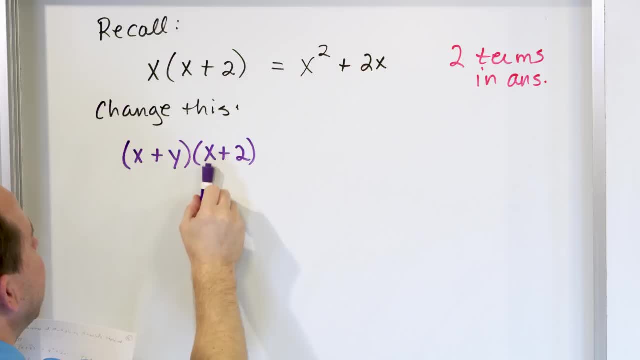 This first guy on the outside has to multiply into the X, And then this first guy also has to multiply into the two, because basically you just pretend the Y's not even there. because basically you just pretend the Y's not even there, there at all. if there were just an x out there, then you would just do whoop, just like this. 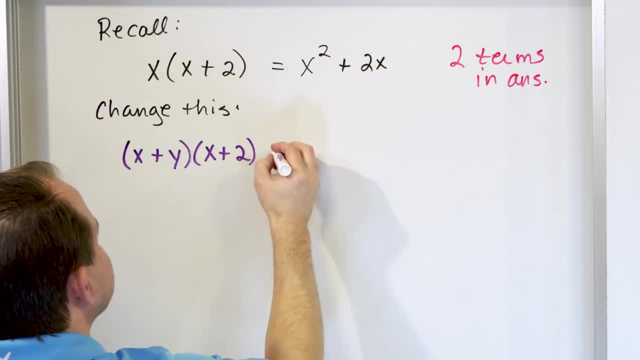 multiply times each interior term. So let's write those down. If you just multiplied x times x, you would get x squared. And if you just multiplied x times the 2,, you would get the 2x. Okay, great, But you can't stop there, because obviously you have something else out here. 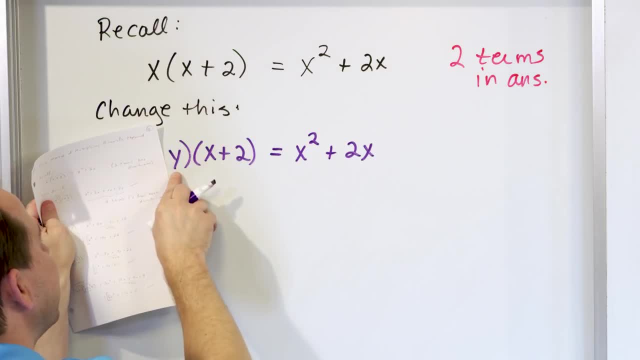 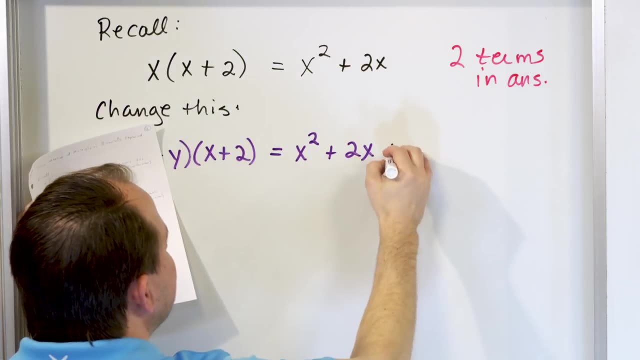 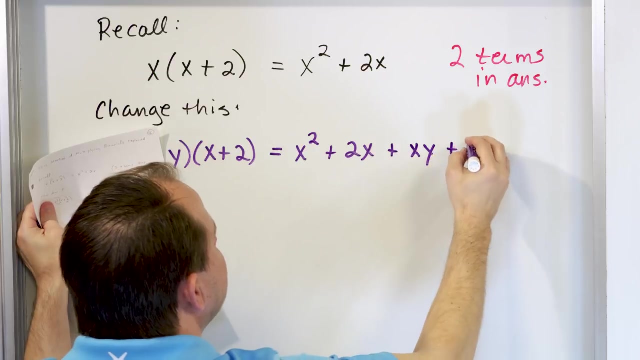 If you were to cover up the x and if you were only multiplying by y, you would multiply y times, also, each interior term, which would be y times x. You could call it yx, but I'm going to call it xy, just because I like to write it that way instead. And then y times 2 is going to be 2y. 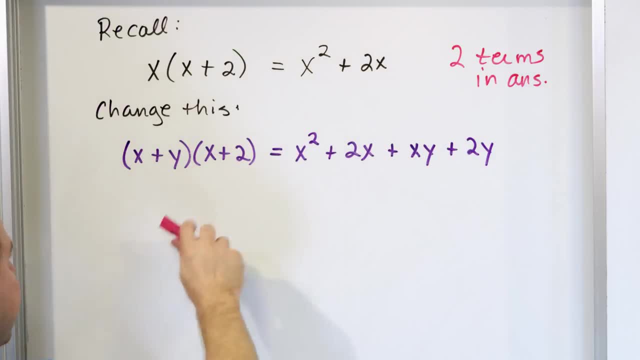 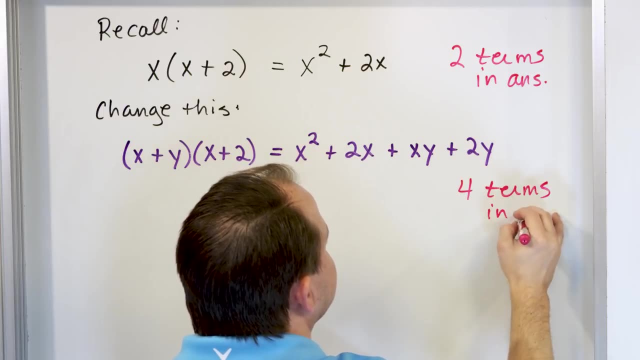 And notice that what you've done, when you've done this here, is there are now no longer two terms in the answer. There are four terms in the answer, right? The reason that there are four terms is because you're multiplying two terms on the inside of something. 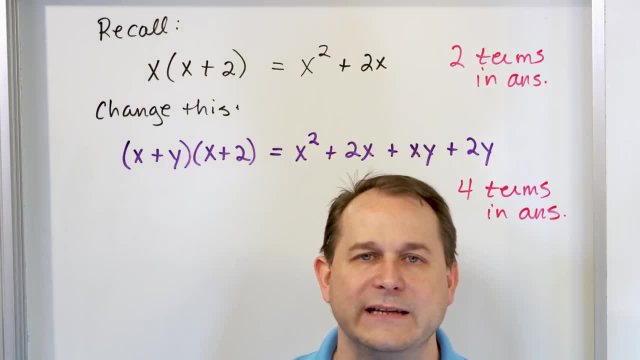 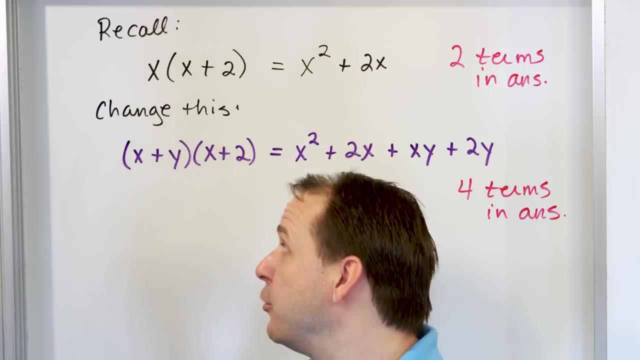 times two terms on the outside of something. And in order to get a complete multiplication you have to multiply: every term on the outside times every term on the inside, And then, on the other term, every term on the outside here times every term on the inside. So because there's two, 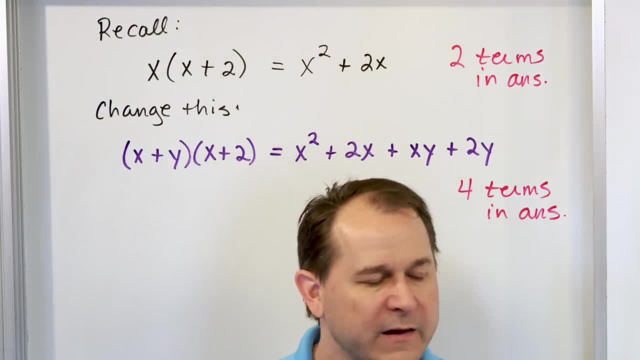 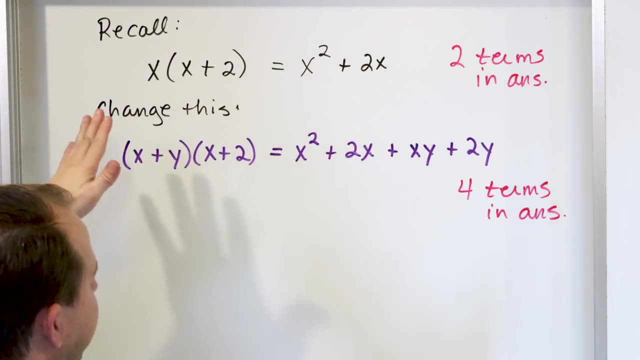 terms in both places, you get four terms in the answer, right? So this is actually the answer to this multiplication. We haven't talked about FOIL yet. I'm going to get to that later, Don't worry about it right now. For now, I want you to know that whenever you're multiplying this times a, 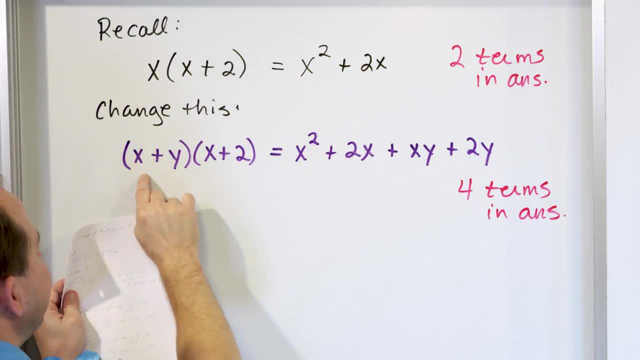 you just take the outside guy. It has to be distributed to each term on the inside. In fact, what I usually do is I remind you of that by drawing an arrow here to say we're multiplying that times that, And then we're multiplying that times that, And on the bottom I'll draw an arrow. 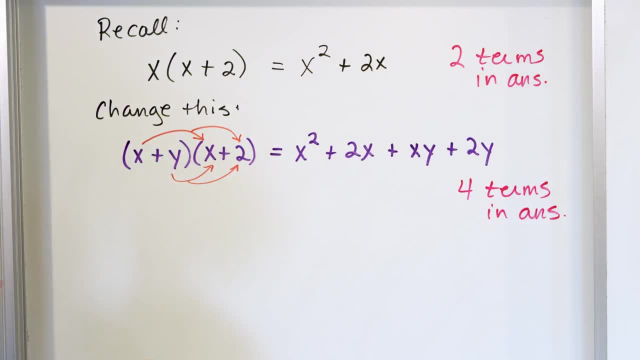 here, showing you that I'm multiplying the y also by both terms. That's why you get four terms. So these two come from the first two multiplications of this one And the last two come from these two multiplications of that one. That, in a nutshell, is how you multiply. 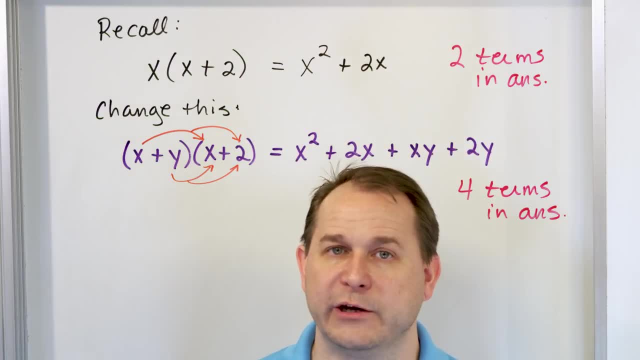 You multiply two binomials together. Two binomials together. Now I'm going to give you a little bit of a preview. I don't want to get into the details of it right now. I'm going to get into it in a few. 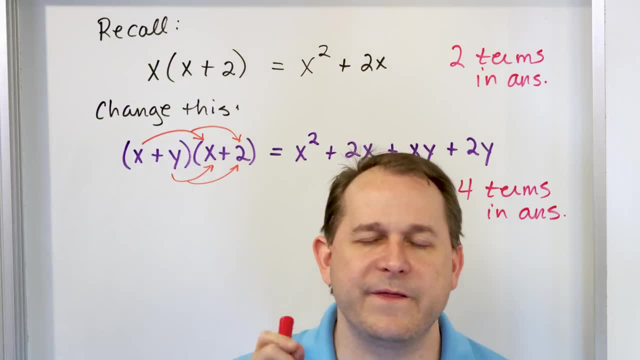 lessons, But I want to give you a preview. What do you think you would do if what you were multiplying on the outside did not have two terms? What do you think you would do if there was a third term out here, like x plus y plus z, all out here? Well, you would have x times these two terms. 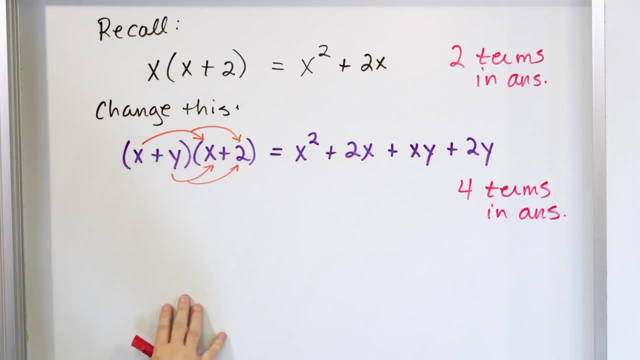 And then you have z times those two terms And then you would add them all together, So there wouldn't be four terms in the answer, There would actually be six, Because you'd have three times two And that would give you six. So you see why I like to teach it this way, Because I'm showing 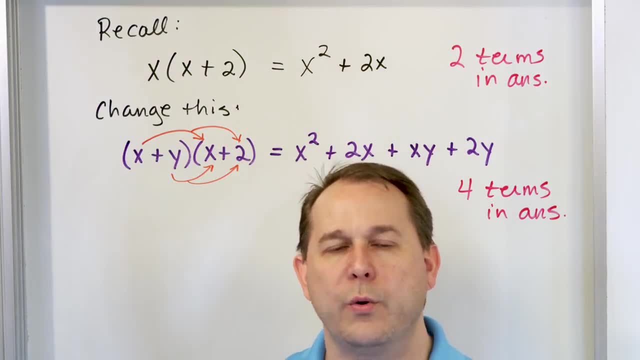 you logically how what we're doing is a direct result of what you've already done with distributing regular terms. So now you can multiply this And you know what's happening. You're distributing each term And then later on, if I give you a much, much more complicated expression, you're 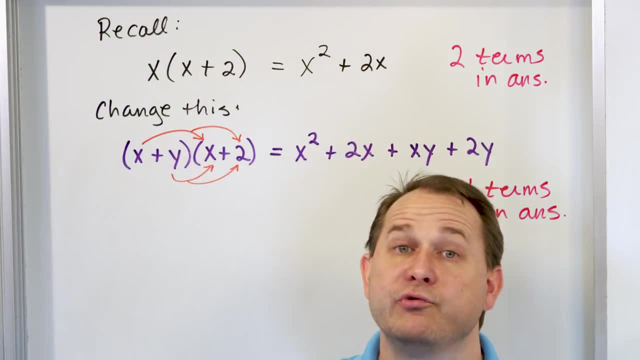 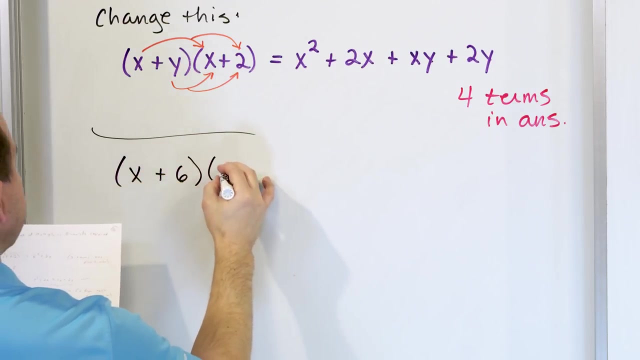 going to get a lot more complicated expression. Then you can just do it, Because you know that every term has to go in and multiply by every other term. So then let's take another example. We're going to fly through a few examples now to give you a little more practice. What if I have x plus 6 multiplied by x plus? 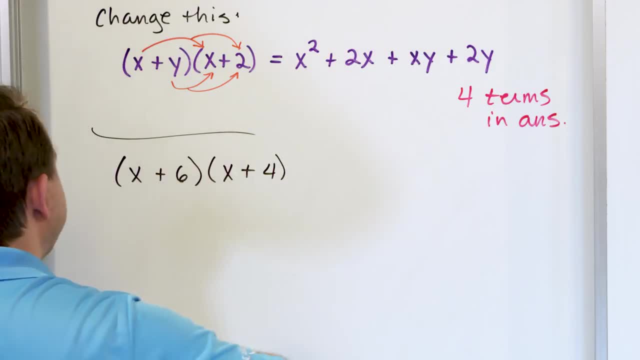 4?? Well, it's the same kind of thing. I have to take the x and multiply it by the first term, And then I have to take the x and multiply it by the second term, which is going to give me what. 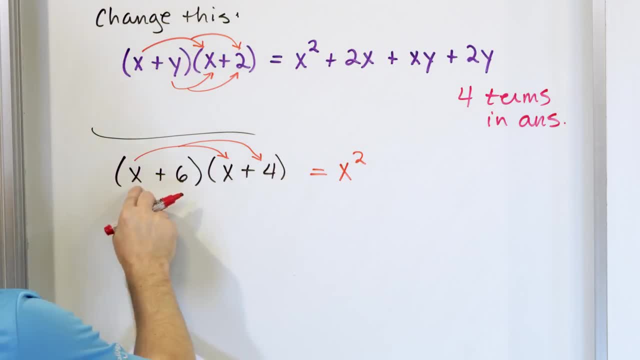 x times x gives me x. squared x times 4 gives me 4x. We generally write the number first, And then I'm going to have this secondary term multiplied in by each of these as well. 6 times x is 6x And 6 times. 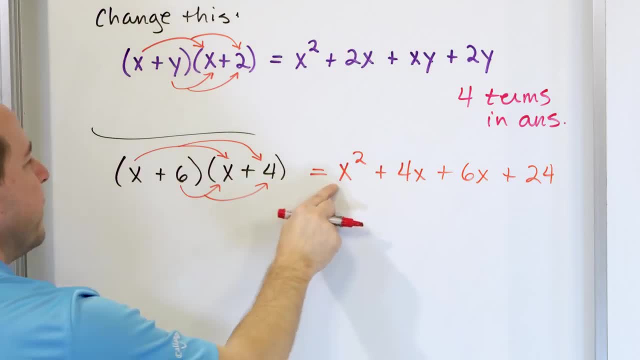 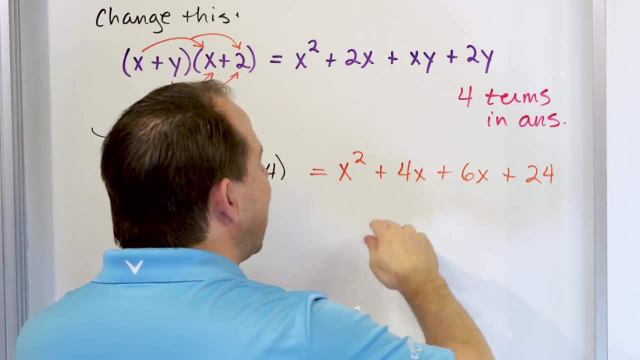 4 is 24.. Now notice: I got four terms here, just like I did here. The only difference is, when I look at this, I realize I have a 4x and I have a 6x, So actually I can combine. 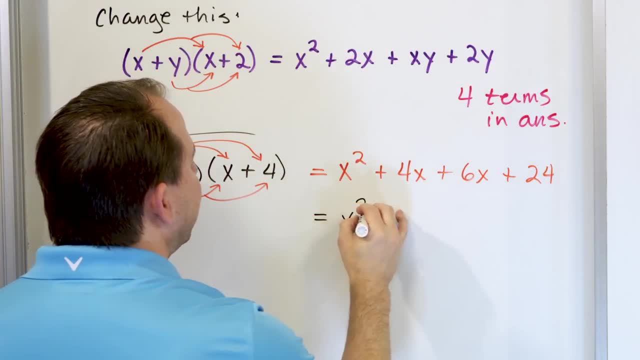 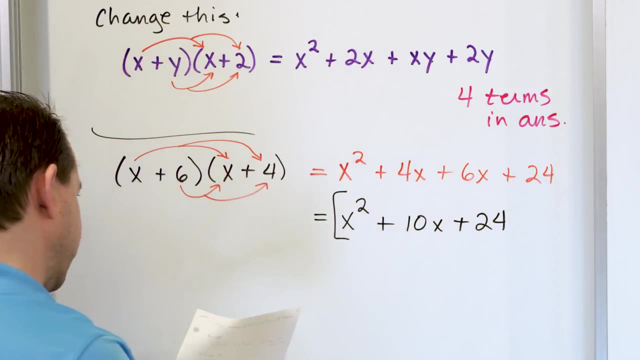 these two and add them, Because they're like terms. So I'll have x squared plus the 4x. This will be 10x plus 24.. And that will be the final answer: x squared plus 10x plus 24.. 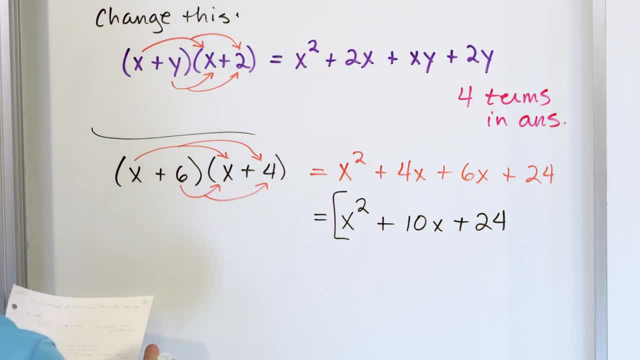 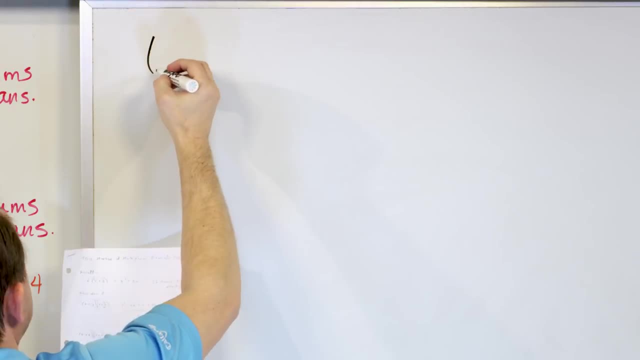 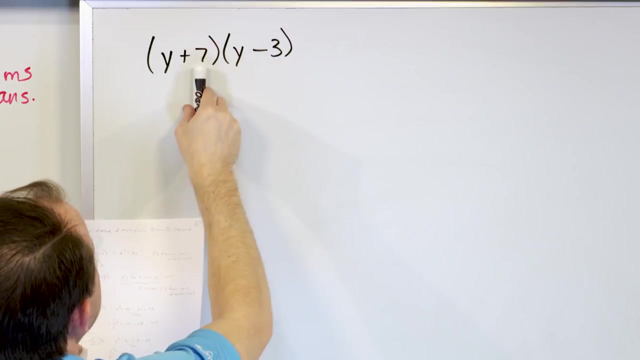 All right, Let's do one more on the next, Let's do a few more on the next board, and then we'll talk a little bit about FOIL. All right, So then for the next one, just to get some more practice: y plus 7 multiplied by y minus 3.. So you pretend the 7 isn't here. 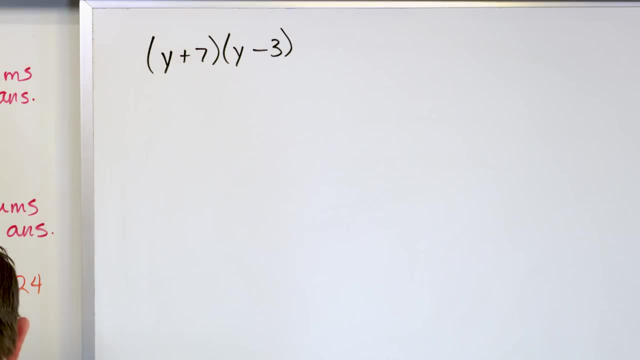 at all, And I'm going to stop drawing my arrows for every problem. This will probably be the the last one that I do. But this y needs to be multiplied by each term on the inside, distributed in as you would guess. So then, what we're going to have is y times y is going to give. 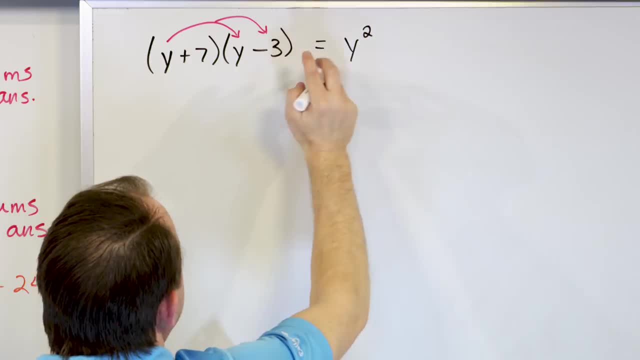 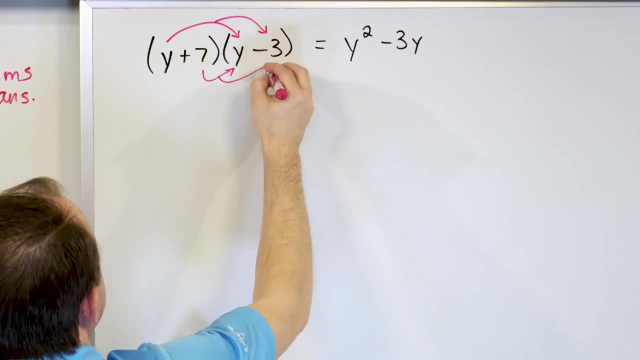 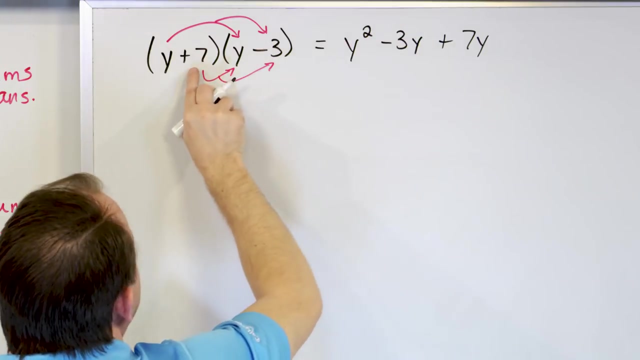 you y squared y times a negative 3 is going to give you negative 3y. But then, after you're done with that, to complete the multiplication, the 7 has to be multiplied here and it also has to be multiplied by there as well. So what is 7 times y? It's 7y. What is 7 times negative 3?? 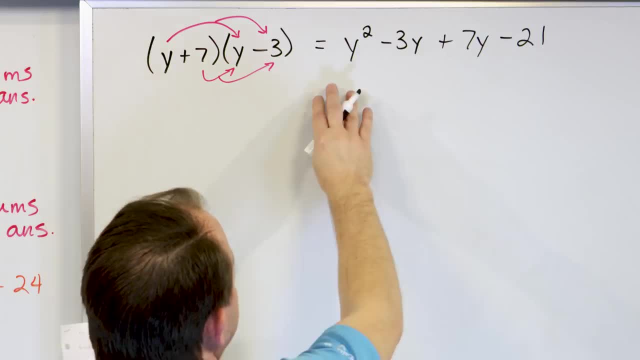 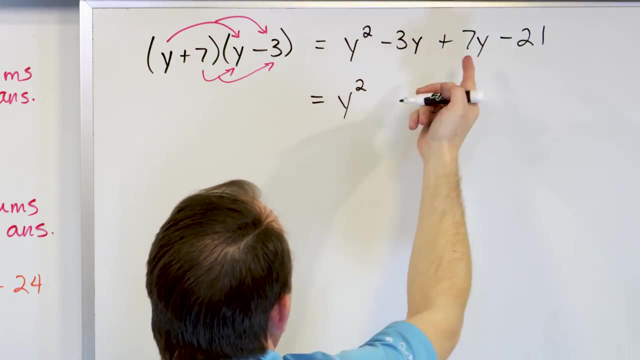 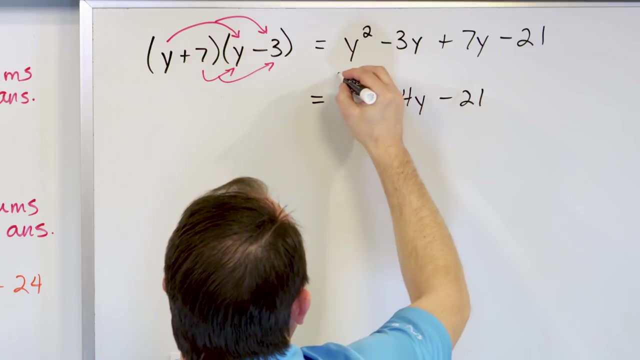 That's negative 21.. Then I say: I'm done with four terms. However, I can add these together. They're like terms, So I'll have y squared What is negative: 3 plus a negative- I'm sorry- plus a positive. 7 is plus 4y, And then I'll have a minus 21 here on the end. y squared plus 4y. 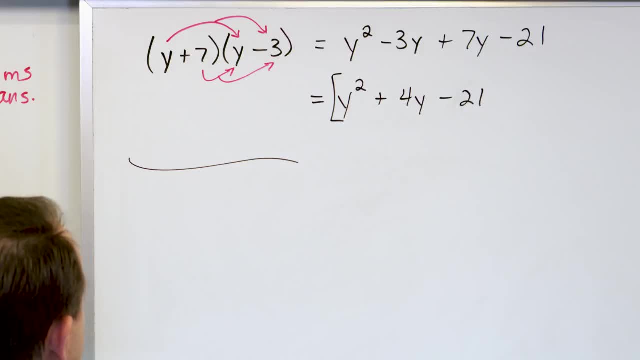 minus 21.. That's the final answer to that problem. All right, let's take it a little bit more complicated, just a notch. Not too bad, though. What if we have 3y plus a negative 7? That's a positive 7.. And then I'll have a minus 21 here on the end. 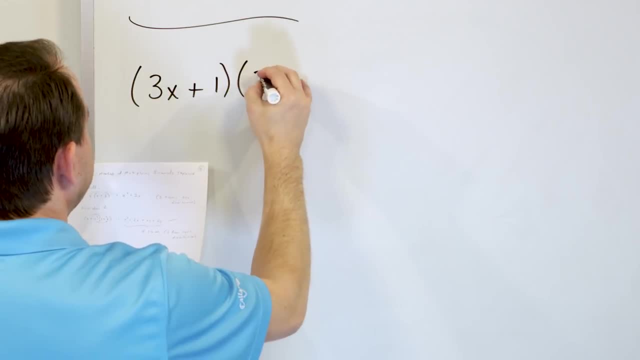 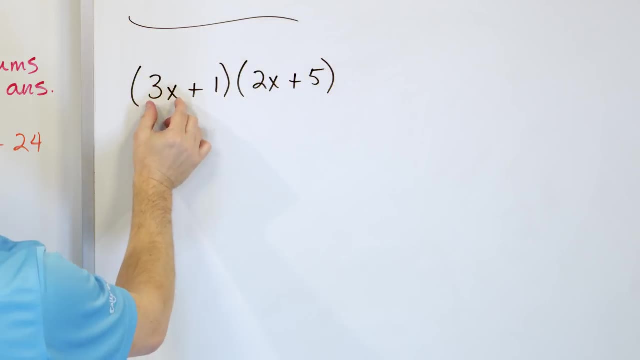 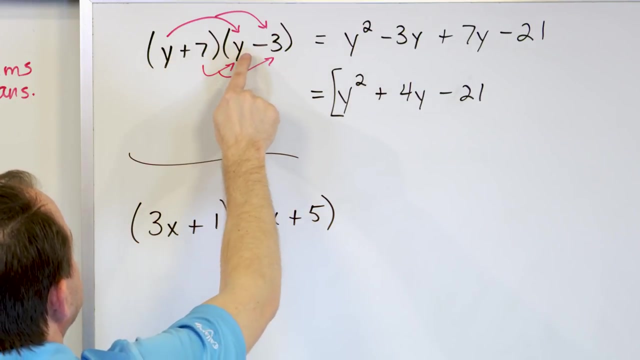 3x plus 1 multiplied by 2x plus 5.. So it's going to be the same thing. The only difference is the first term here actually is three times a variable, The first term here is two times a variable And, in fact, all the other problems. we just had single variables and single digit. 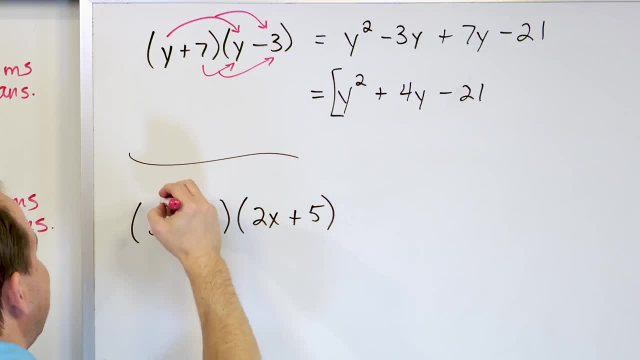 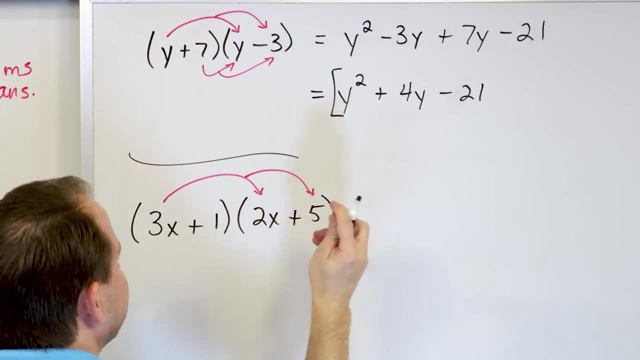 things everywhere, But exactly the same thing applies. We have to take this 3x and we have to multiply it times both of those guys over on the other side. So what is 3x times 2?? It's going to be 6.. And what is x times x? You add the exponents, giving you x squared. 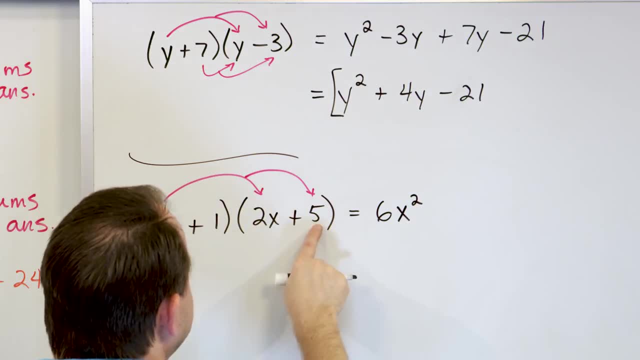 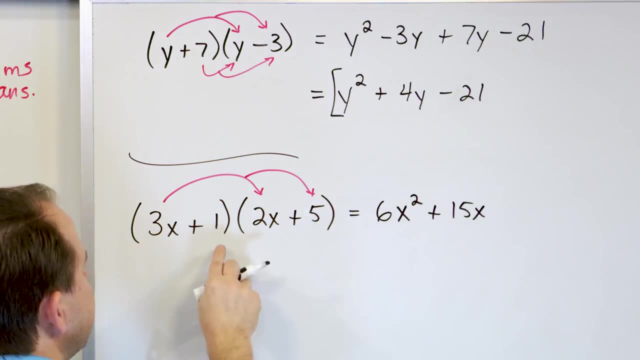 Now you have to take this and multiply and distribute into the other guy, which is 5.. 3 times 5 is 15.. And the x is still multiplied 3x times 5, so it's 15x. Then we'll take the 1 times. 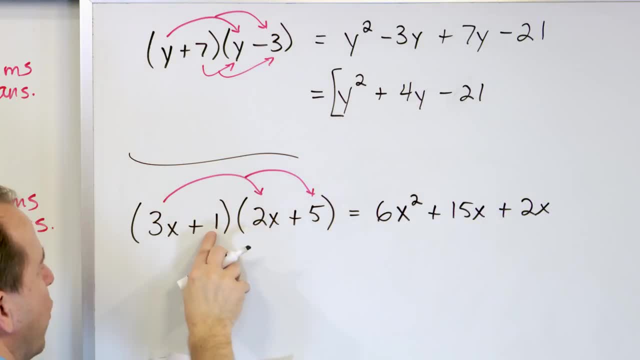 the 2x giving you 2x, And we'll take the 1 times the 5, giving you a 5.. And then we realize we can combine these like terms. So we'll have 6x times 2x And we'll take the 1 times the 5, giving you. 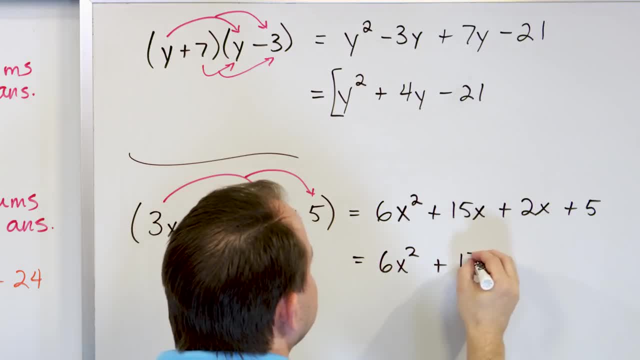 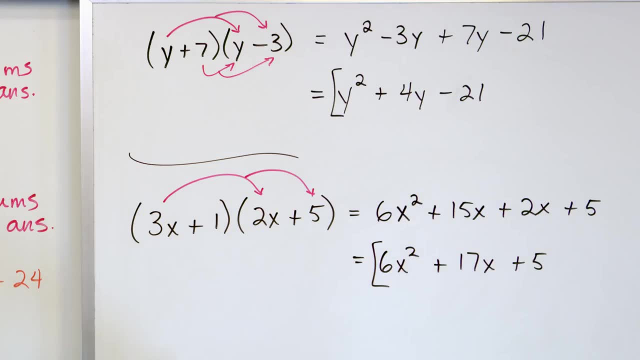 6x squared, What is 15 plus 2?? It's 17x, And then the 5 comes along for the ride. So 6x squared plus 17x plus 5.. All right, So what I want to do is first of all call your attention to the fact. 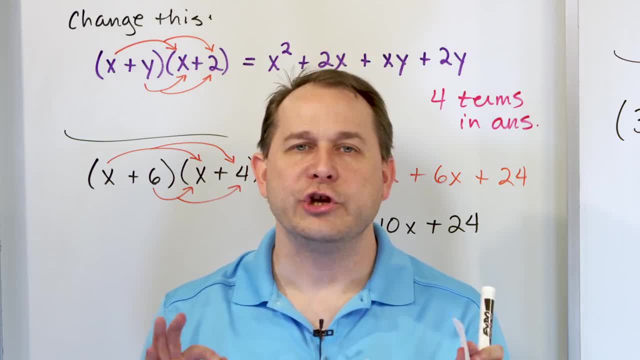 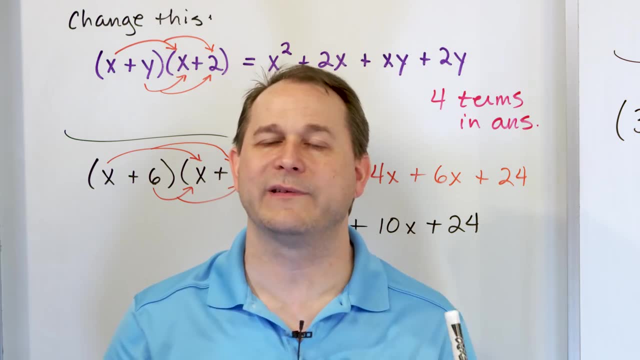 that we talked about how to multiply these binomials together using nothing more than an extension of what you already know- how to distribute things on the outside- And now you know that when you have two terms linked together, then they have to be each multiplied by everything. each distributed by everything. So what I want to do is, first of all, call your attention to the fact that we talked about how to multiply these binomials together using nothing more than an extension of what you already know: how to distribute things on the outside. And now you. 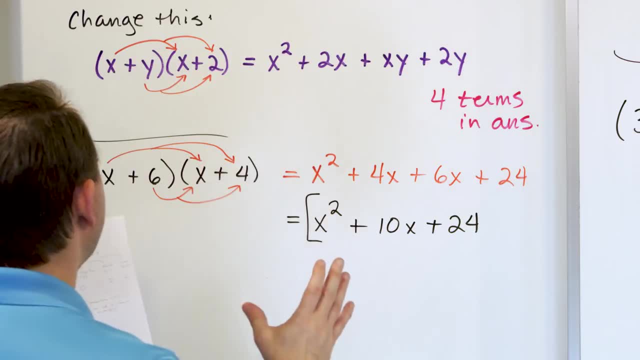 know that when you have two terms linked together, then they have to be each distributed in to the following term. Now let's zoom in to one of these examples a little closer. this one here: the x plus 6 and the x plus 4.. I'm going to do that on the other board And we're going to 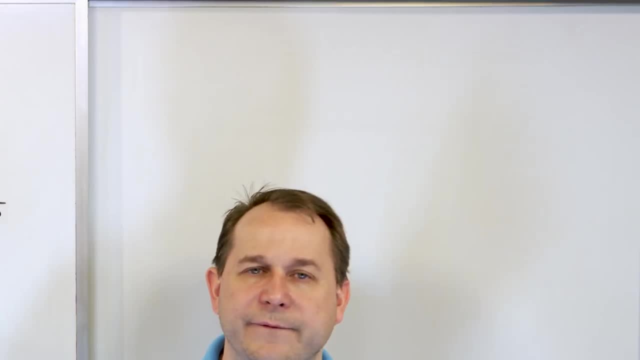 talk a little bit about FOIL, And you're going to see, the punchline is that the FOIL method of multiplication, which I teach you in class without telling you what it's for, is exactly what we've just done here, So you're really learning nothing new. Let's examine one of these a little bit. 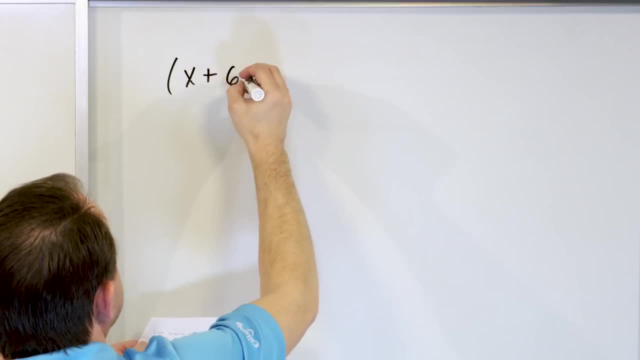 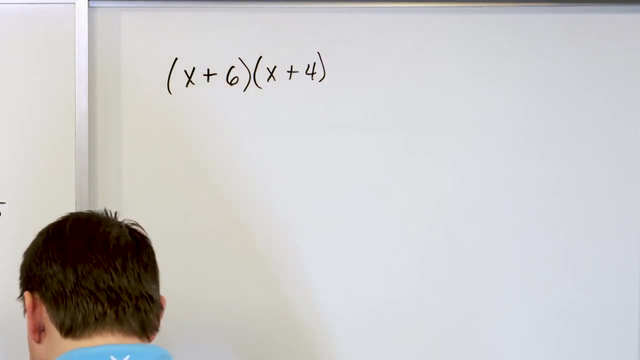 further. Let's say we have x plus 6 multiplied by x plus 4.. So I'm choosing this one because I'm we've already done it before, so the x times the x. let me go ahead and for this one case i'm going. 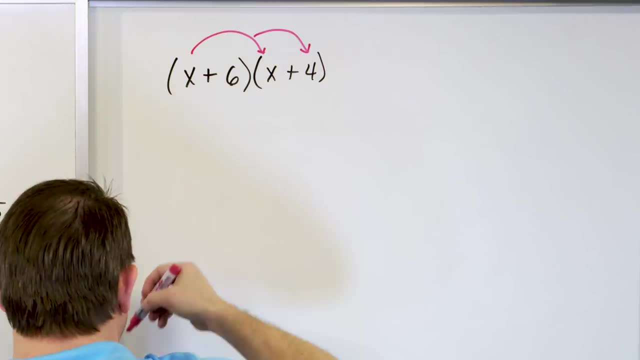 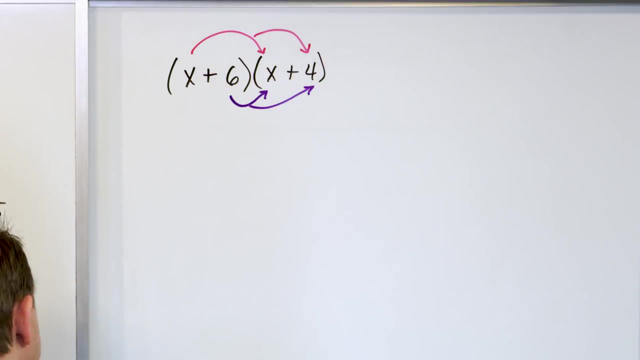 to go ahead and go ahead and do this. draw my little arrows because i'm going to be coming up that direction. i'm going to do a different color for the bottom ones, like this: so when we do the uh first, guy x times x will give me x squared. and then six uh times f- sorry, x times the other. 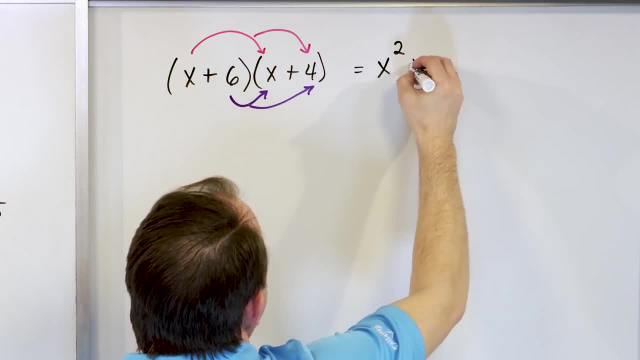 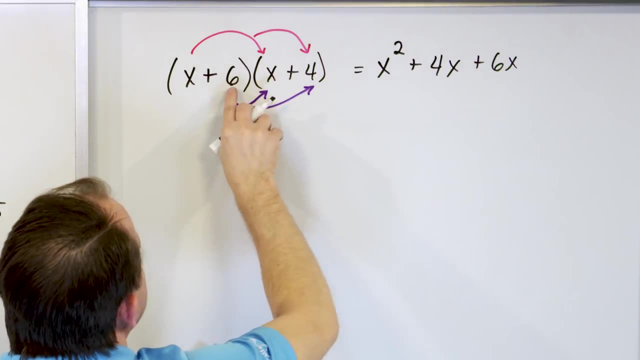 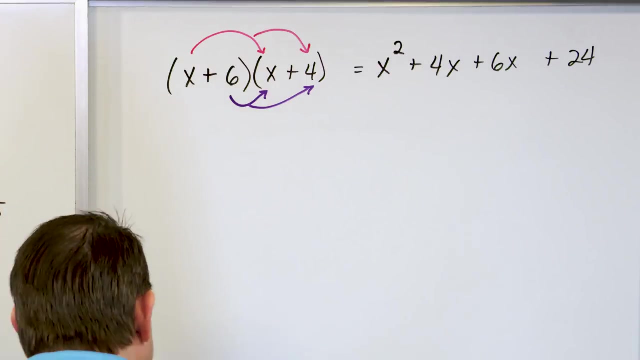 guy over here will be four x, six times, or x times four is four x. then we have the six. the second term times x will give you six x, and then the six times four is twenty four. let me just double check. i didn't make any silly mistakes so far, all right, notice what we've done. i've explained it to you. 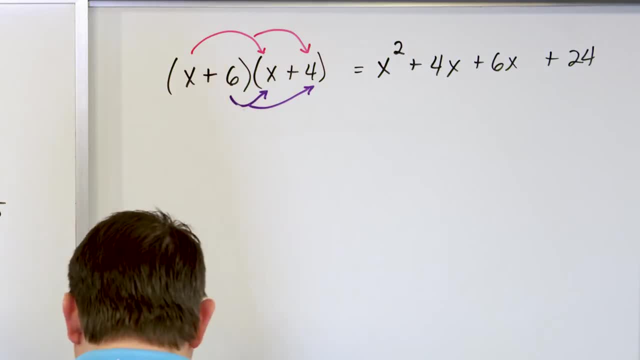 as distributing n from the outside, which is all correct, but notice that there's an easy way to remember this for people that don't learn it: the. what i consider to be the right way is that the first thing that we multiply together is the first terms. in other words, this is the. 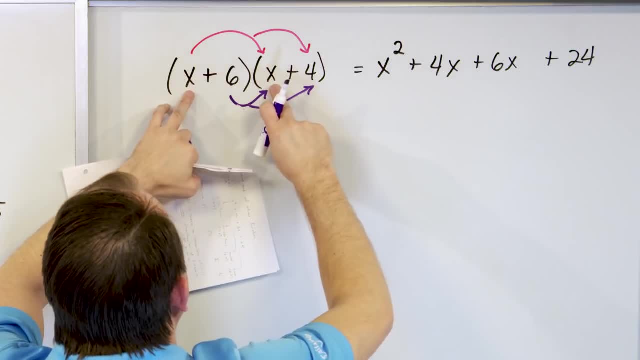 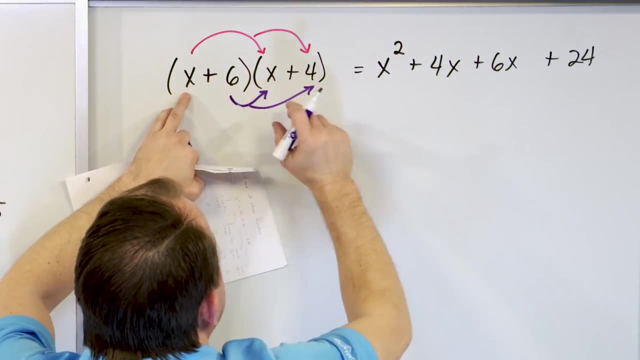 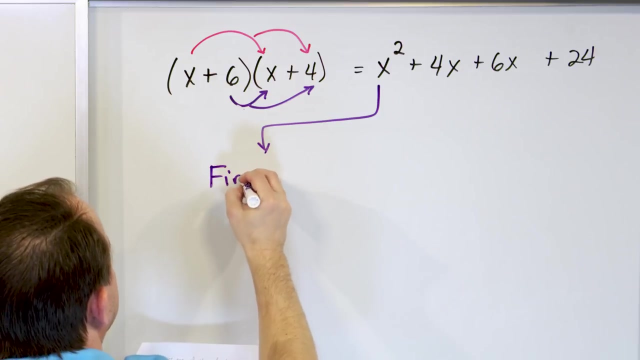 binomial. this is another binomial, this is the. these are the first terms. the x and the x are what we call the first terms, because this is the first term of this one and this is the first term of this one, right? so this guy, i'll go ahead and draw it out here. this is called first terms. 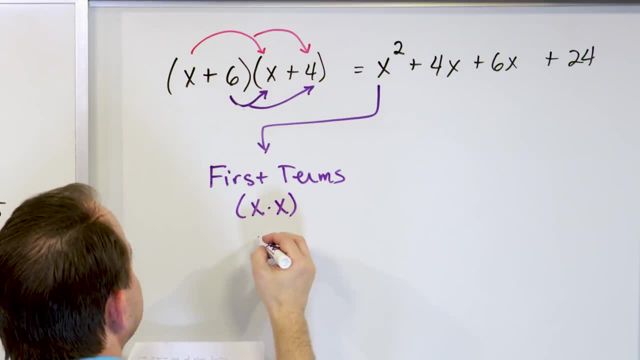 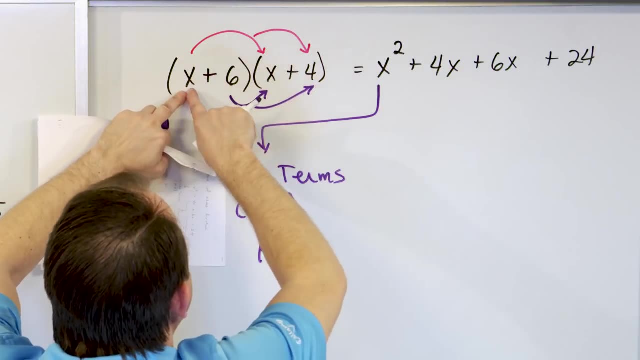 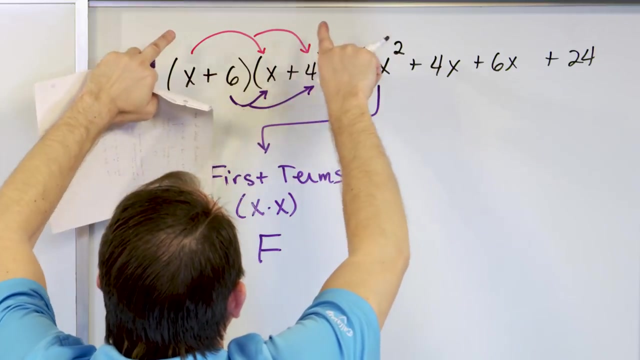 and that was x times x, right, and so, because it's first terms, we're going to put an f there and then after that we multiplied x times four. but this is the- uh, outside terms, right? so these are the first terms of each guy. this x times the four. these are the outside terms. they're on the outside most part of the parentheses. 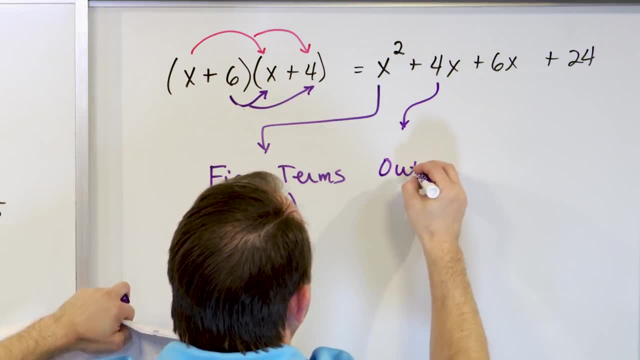 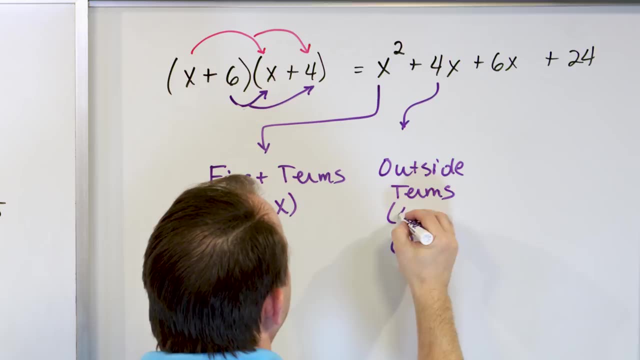 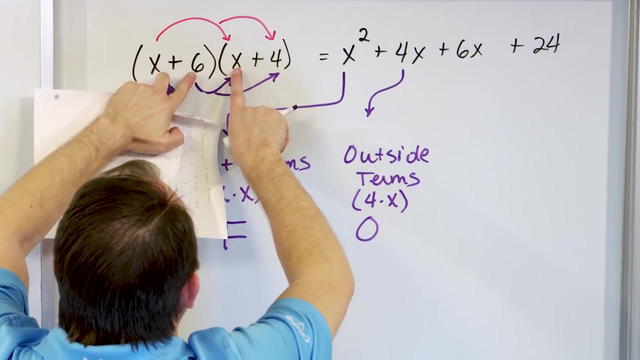 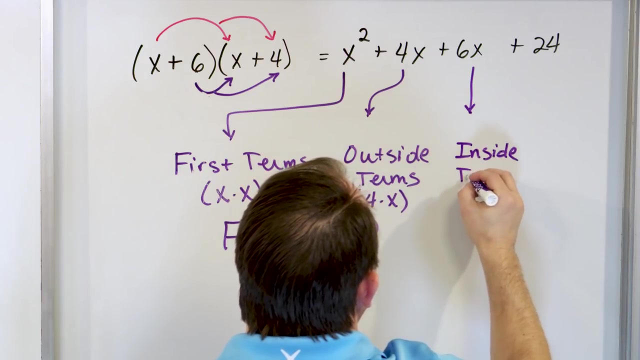 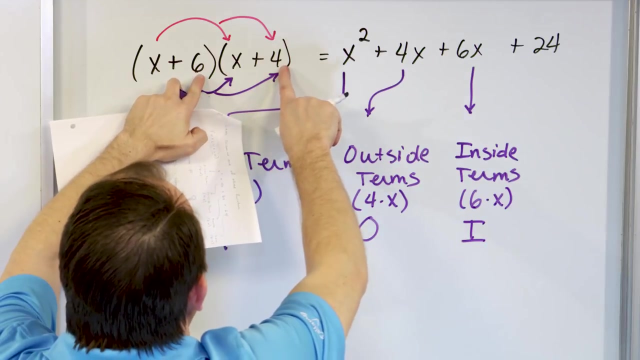 so this guy here is what we call outside terms. so we call that o and that was, uh, four times x. all right, then notice that we multiplied the six times the x. these are the inner terms, the most inside, most terms. so we label this inside terms six times x and we call that capital i. and then these are the last terms, the last terms. 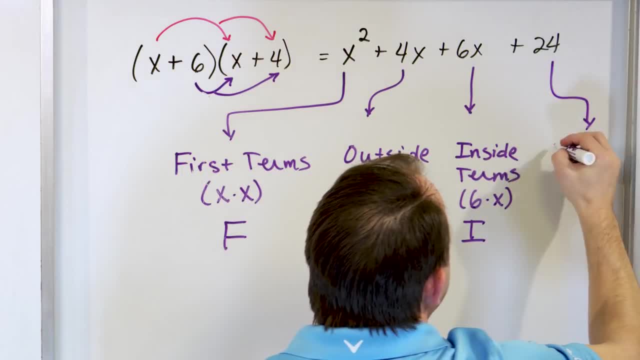 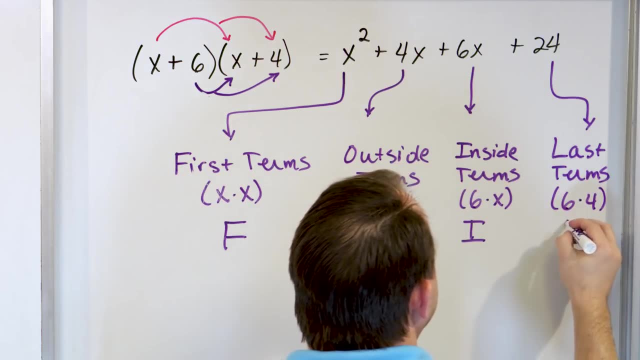 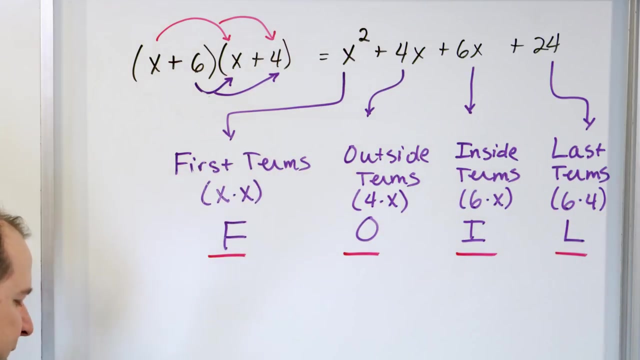 in each of the two binomials six times four. so we label that the last terms and it was six times four and it was last. so this is the famous foil method of multiplication: first, outside, inner, last. typically, what most algebra teachers, what most algebra books are going to do, is they're going: 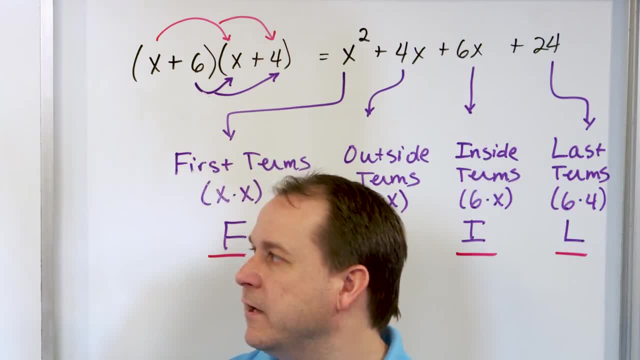 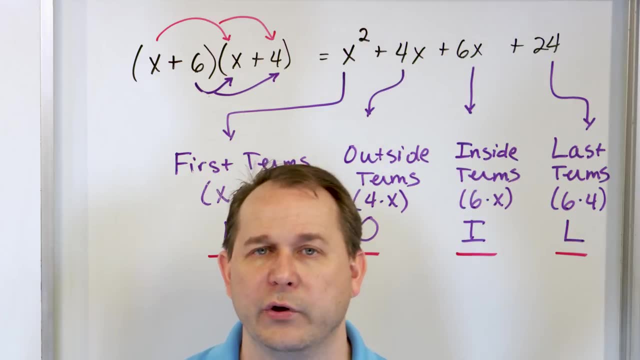 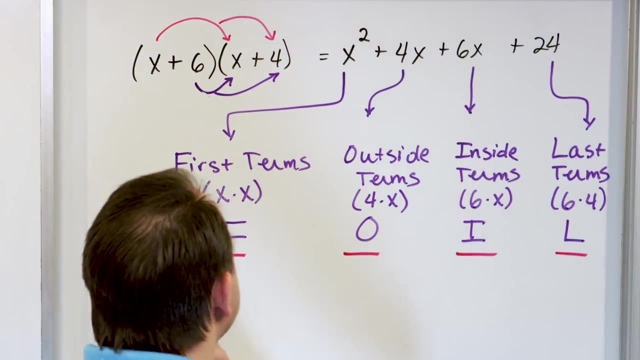 to say: hey, when you're multiplying two binomials together, like you know, in this case it's x plus four and x plus six- when you're multiplying two binomials together, follow this recipe called the foil method. foil means first, o means outside, i means inner and l means last. so the first. 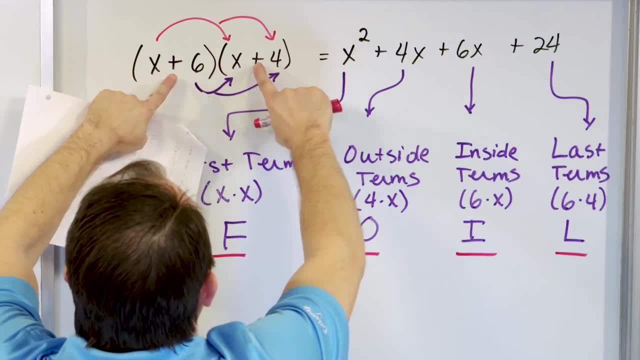 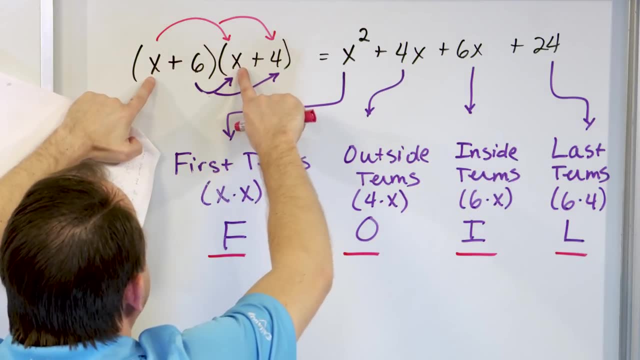 terms are these two terms, the outer terms are these two terms, the inner terms are these two terms and the last terms are these two terms. and all you have to do is first multiply the first terms together, giving you this the outside terms together, giving you this the inside terms. 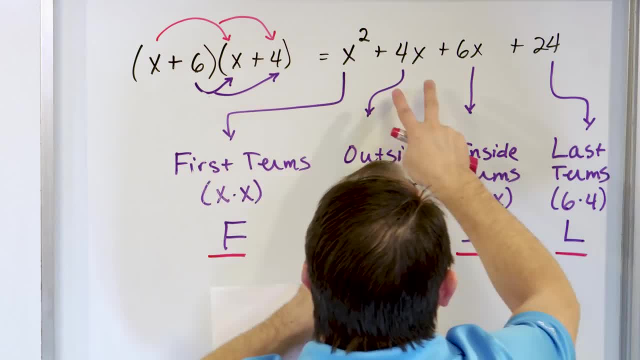 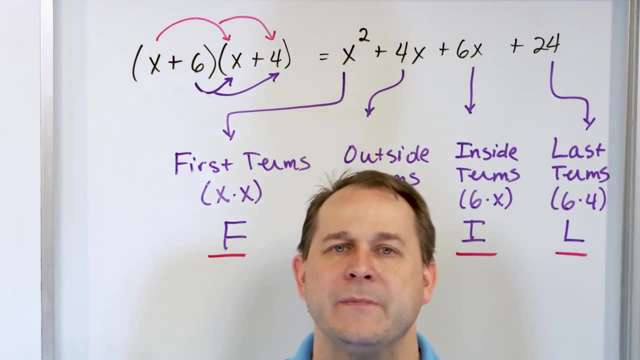 together, giving you this and the last terms together, giving you this. so it's first outside, inner last, and you follow it like a cookbook: first outer, inner last, first outer, inner last. And it works every single time because you write your first outer, inner last multiplications. 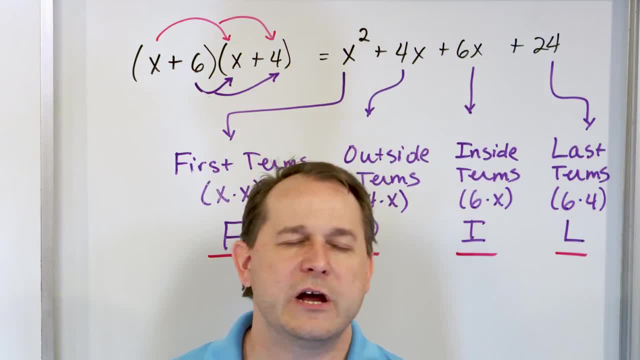 then you add these together and you get the answer, and it's great. There's nothing wrong with using the FOIL method. In fact, as we work more problems in the next few lessons I'll probably refer to the FOIL method subconsciously, because I learned it myself when I learned algebra. 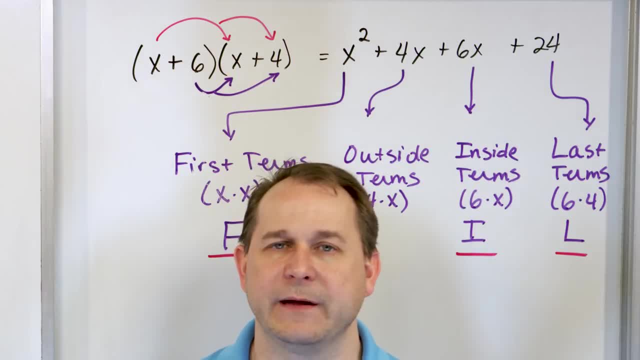 So why am I harping on it? Why didn't I just open this lesson up and say, hey, there's something called the FOIL method. You have to use it. It's because it doesn't help you if any problems exist beyond multiplying binomials together. 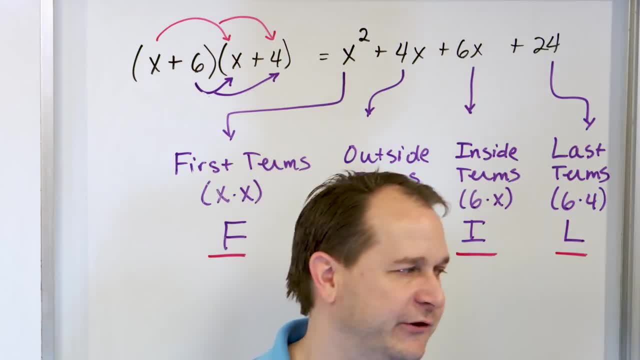 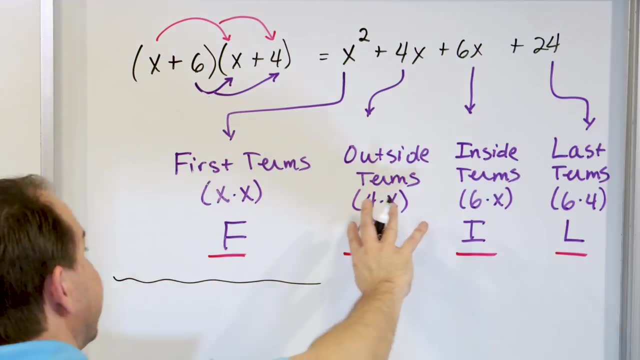 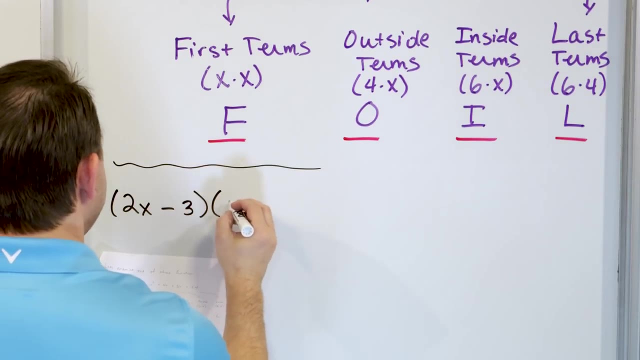 It doesn't help you for any more complicated type of situations. Let me give you an example. Before we get there, let's do one more, as we now know that this is called the FOIL method. Let's take a look at 2x minus 3 times x plus 8.. 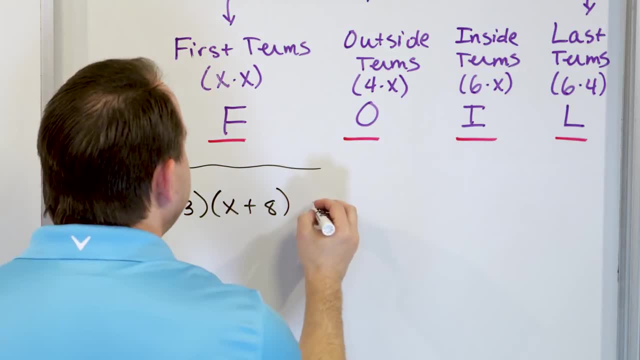 So I've been teaching you just to distribute things in, and that's fine. It's exactly what we've been doing. But you could also just think of the FOIL method. Hey, here's the first terms. 2x times x. 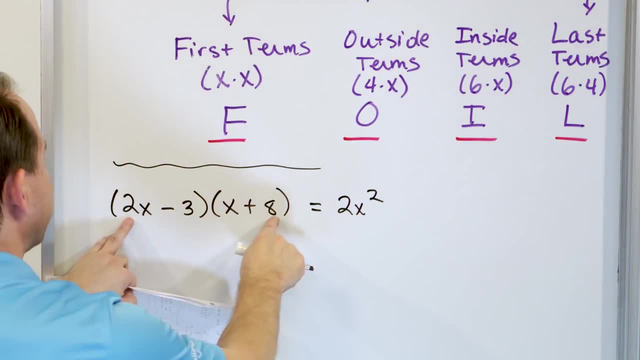 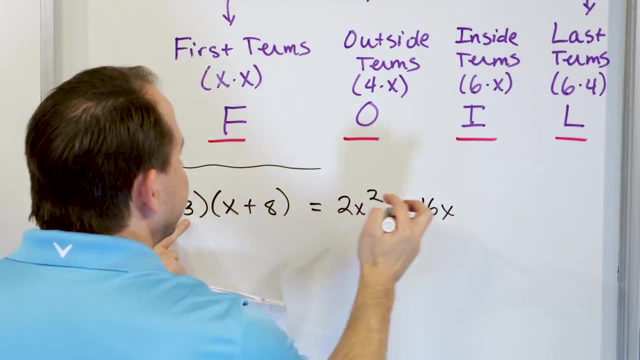 That's 2x squared. The outer terms will be: this is an outer and this is an outer. 2 times 8 is 16, so you get 16x. The inner terms will be negative 3 times x. You have a negative 3x. 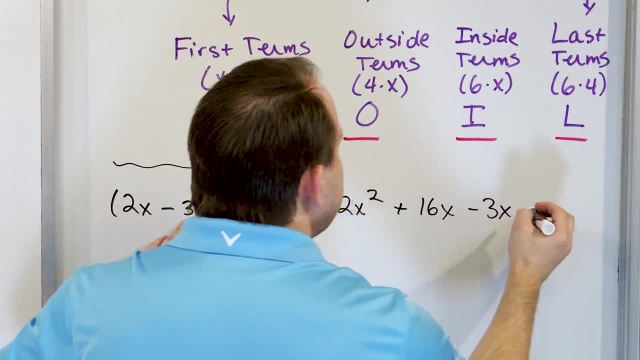 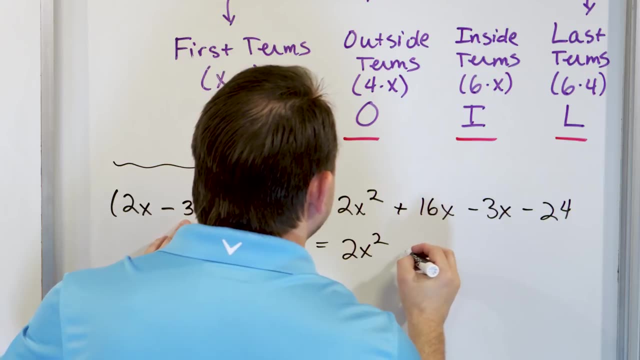 And the last terms will be this: one here: negative 3 times 8 is negative 24.. And then you can add these, so you get 2x squared. What do you get? 16 minus 3 would give you 13x. 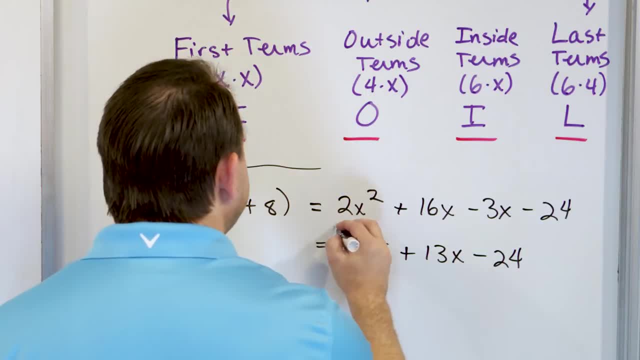 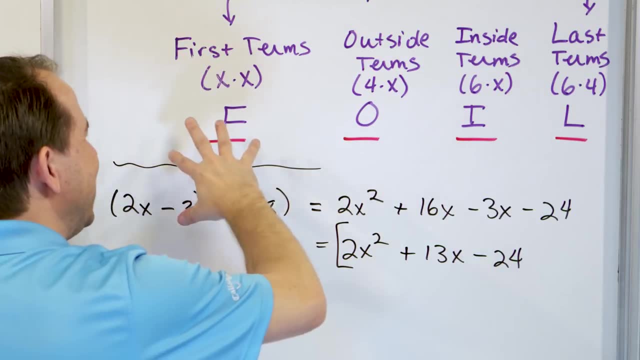 Minus 24.. Let me just double check them right before I continue on. Yeah, that's the right answer. So you see, we did first multiplications, then outer, then inner, then last, which is the exact sequence that I taught you initially. 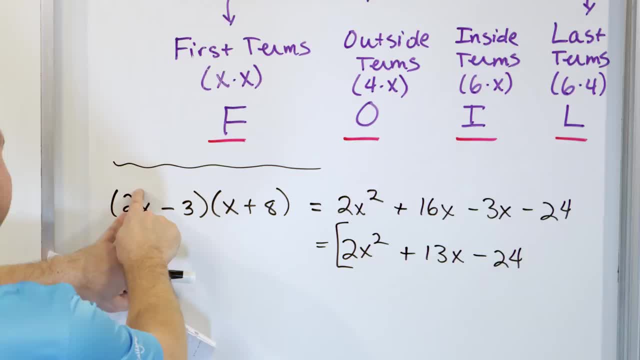 In other words, the FOIL method is exactly what I already told you. The first terms is when you distribute this end. The outside terms is when you distribute this end. The inner terms is when you distribute this end. The last terms is when you distribute that end. 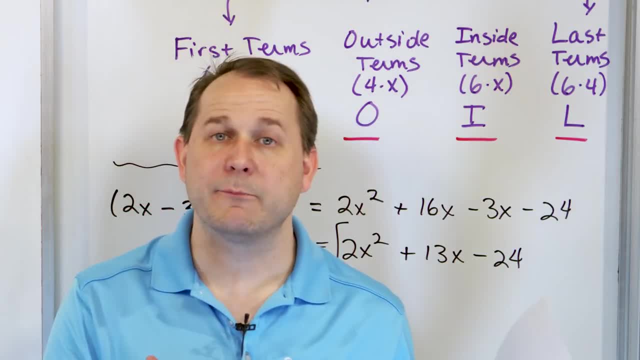 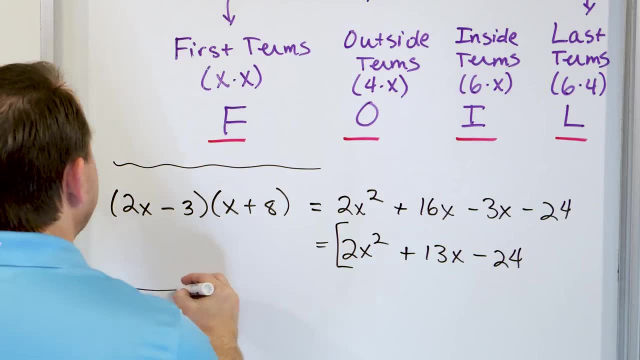 So why am I making such a big deal out of it? It's because people Memorize this recipe first, outer, inner, last, but they have no idea why it works. So then, later down the road, in algebra, maybe I give you this. 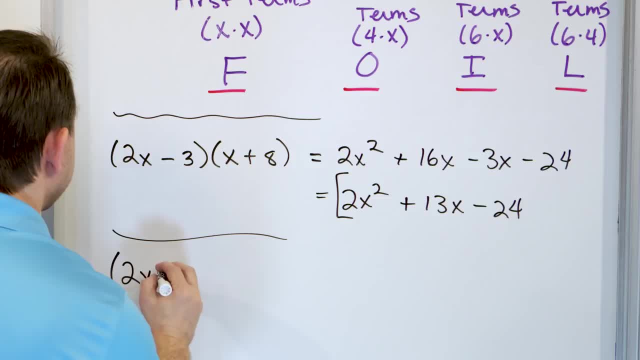 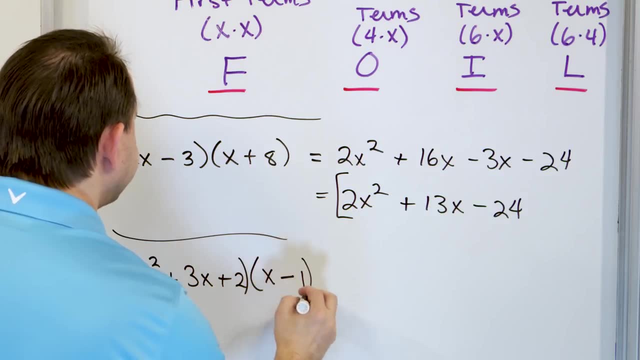 Maybe I give you which we will get to: 2x squared plus 3x plus 2 times x minus 1.. You see, if you've learned the FOIL method: first outer inner last. first outer inner last. 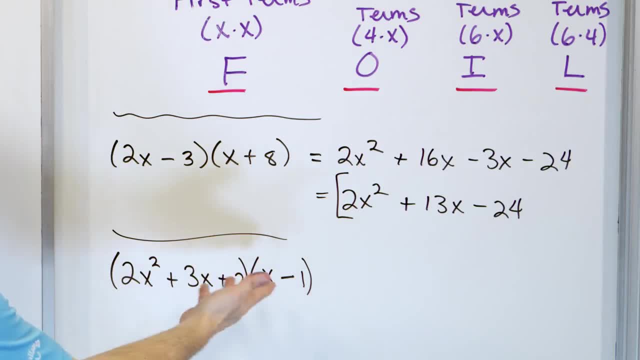 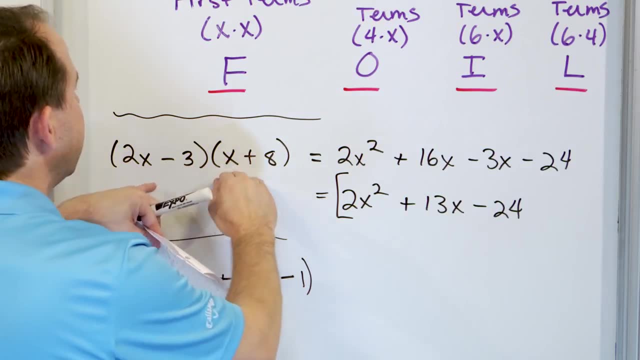 then you have no idea how to multiply this. What's the first terms, What's the outer, inner and last? And then the last term is: how do I do it? You have no idea how to handle anything beyond this cookie cutter recipe. if you just memorize. 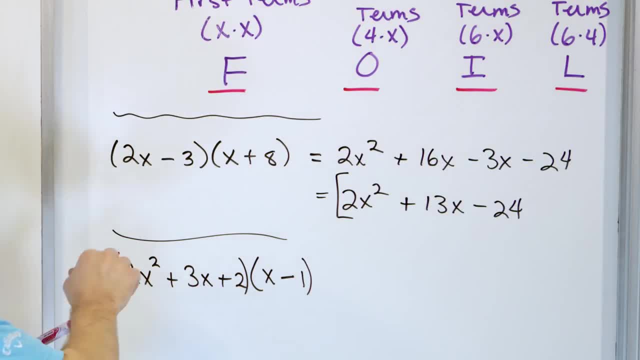 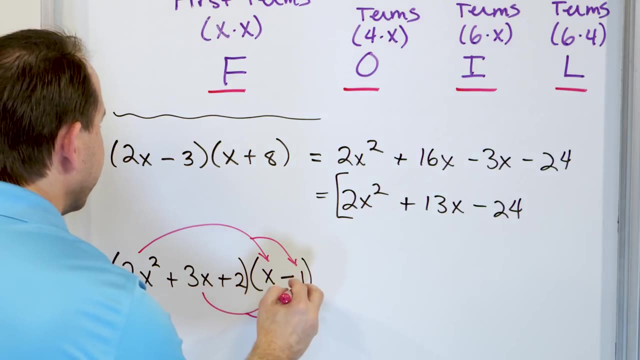 a cookie cutter recipe. But hopefully now you all realize that there's no magic behind how you multiply this together. What you do is you realize this term has to be distributed into each of these, like this: Right, Then, this term needs to be distributed into each of those terms, like this: 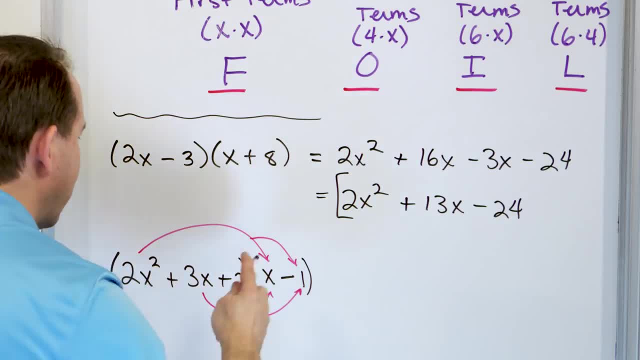 Then that last term, which is kind of hard to show without You getting in the way here, has to be distributed in as well, right? So, even though we're getting a little bit ahead of myself, I think it's really important for you to see 2x squared times x will. 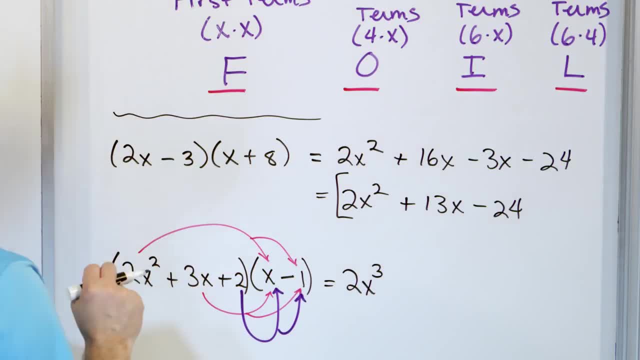 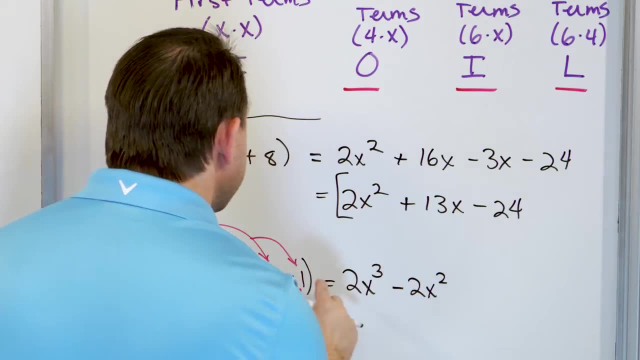 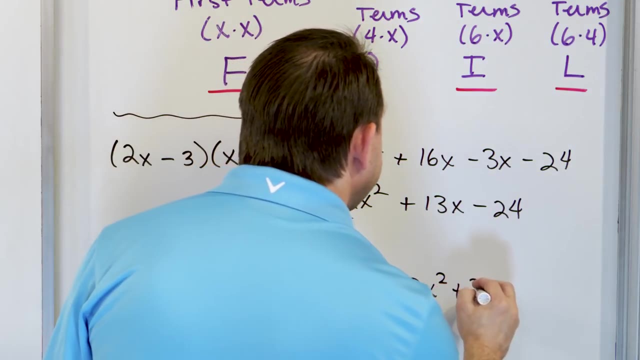 give you 2x to the third power because you're going to have an adding of the exponents. Then 2x squared times minus one will give you minus 2x squared, because negative one times that's 2x squared. Then you move to this term and it has to go into each one as well. 3x times x is 3x. 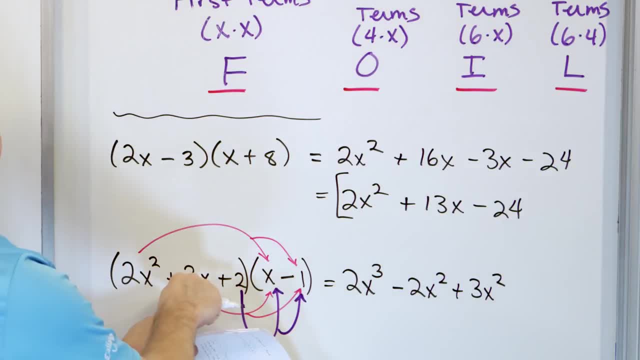 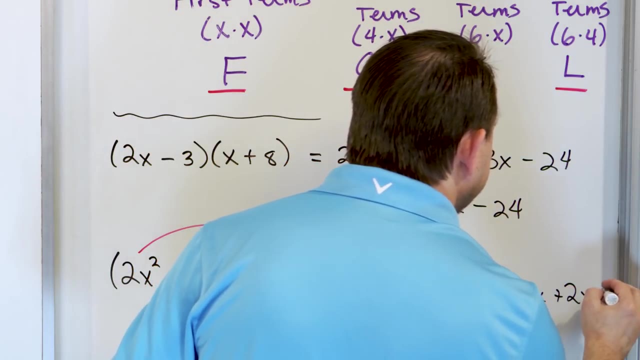 squared, because x times x you add the exponents, Then 3x times negative one will give you negative 3x, right? Then you go to this one, which has to be distributed in: 2 times x is 2x and then 2 times negative one is. I'll have to write it on the bottom, unfortunately. I'll do it. 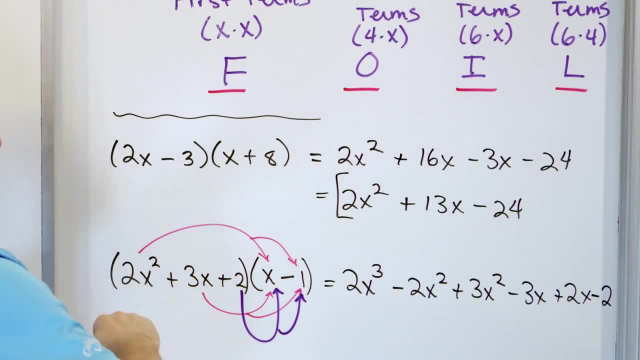 here negative two like this. So you see what's happening. You have now one, two, three, four, five, six terms, Because this one goes boom boom, This one goes boom boom, This one goes boom boom And you 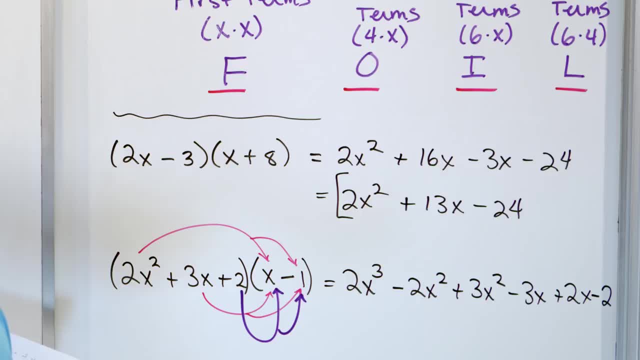 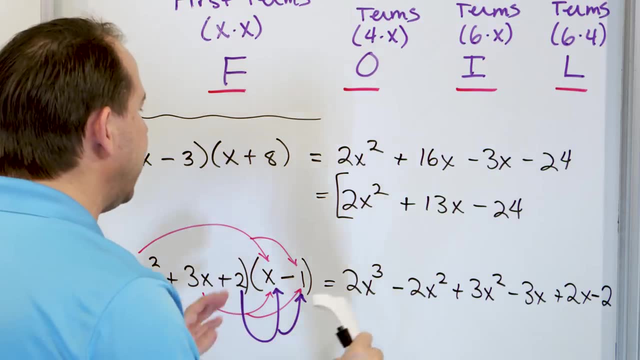 don't ever talk about FOIL, because it doesn't matter. And then if I give you another problem where this one has three terms, then you know how to do the same thing and it works for any multiplication of any polynomials, which we're going to get to a little later. This is a little 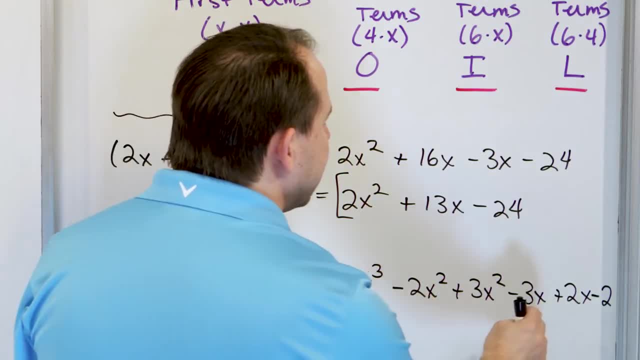 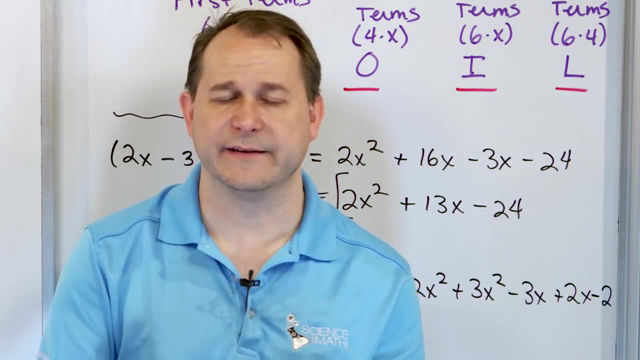 bit of a preview. Of course, I can simplify this by adding these terms. I can simplify this by adding those terms. I'm not going to do it now, because this isn't the point of the lesson. The point of this lesson is that we're learning something called the FOIL method: first outer, inner, last. But it's not a